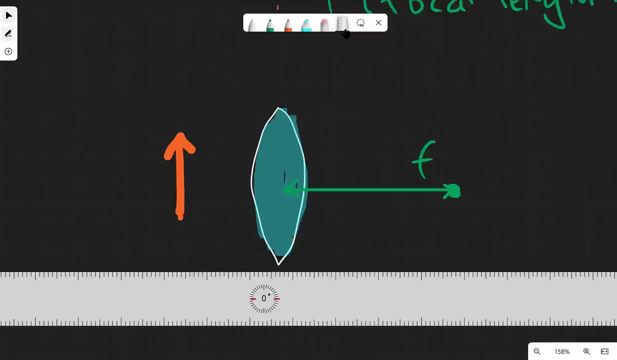 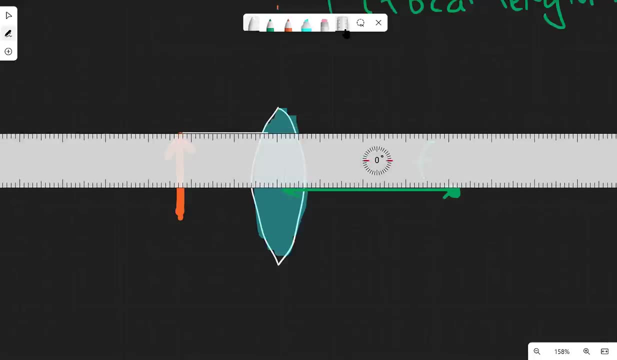 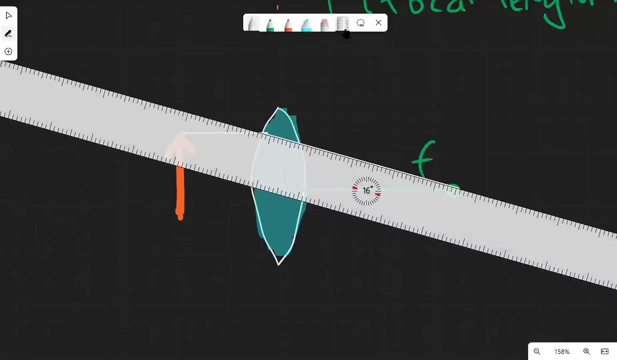 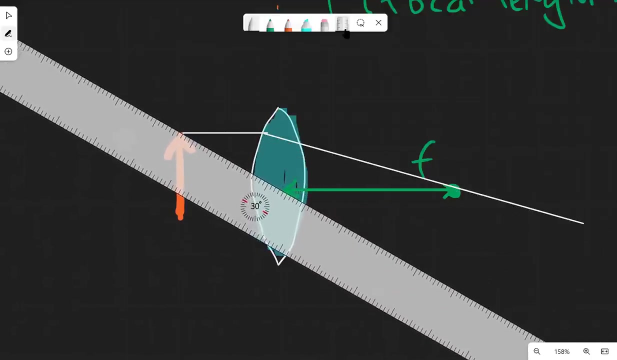 of the focal length. I'm going to be drawing two rays. One of them will be from the object, like so. however, this will then refract and go through the focal point as normal. Now, the other one will be going through the actual center line of the lens that we can just show, like so, to show where my 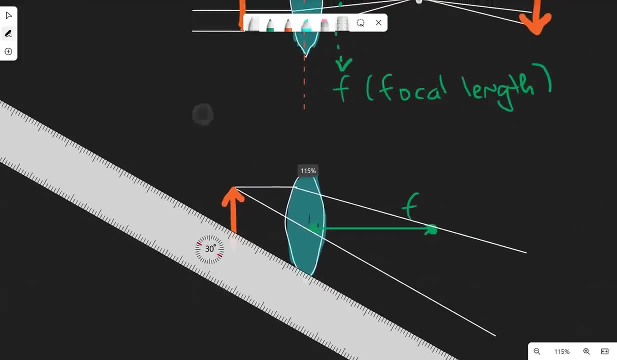 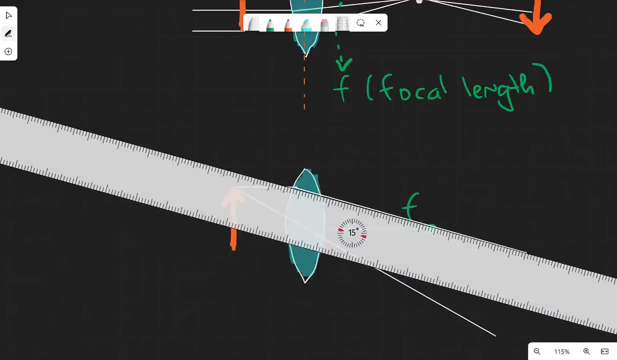 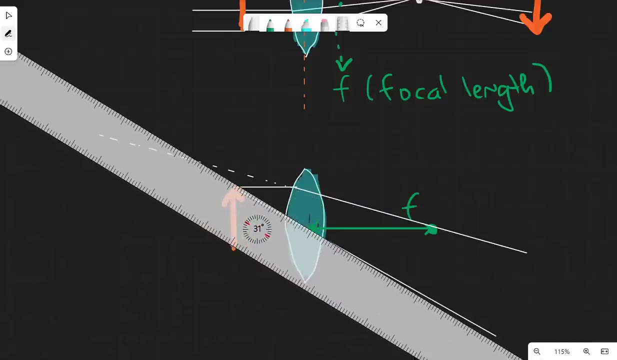 image will be. All I would need to do will be to extend those two rays. So what I'm going to do is I'm going to take this one, then I'm going to extend this, like so, and then I'm going to take this one here and I'm going to extend it like so. There, 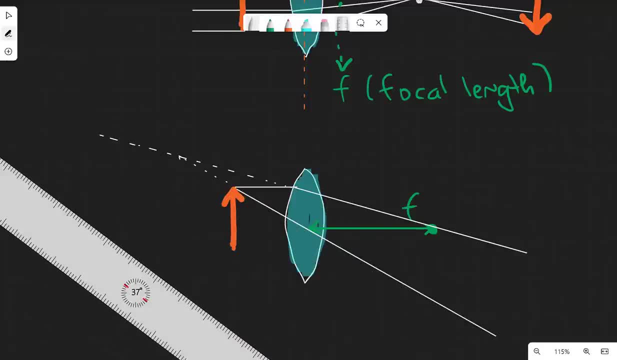 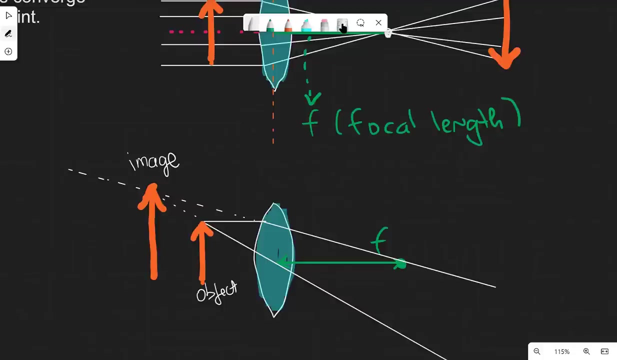 will be an image that will be formed at the point where those two lines meet and, as you can see that this image is on the same side as the object. So this here is my object and this here is my image. To summarize with a virtual image: the image is on the same side compared to the focal length. 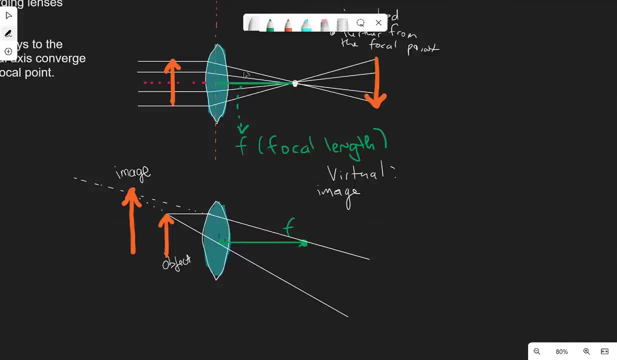 What do I mean with our real image? This was our object And our image was here, whereas on the virtual image, which is this one here, it is the other way. So the virtual, the image, is on the same side, It is not inverted. There's also a formula that will: 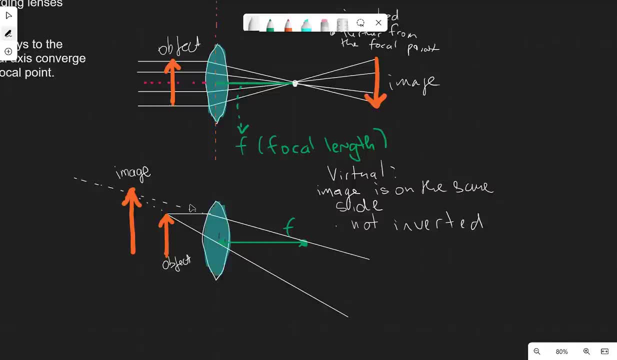 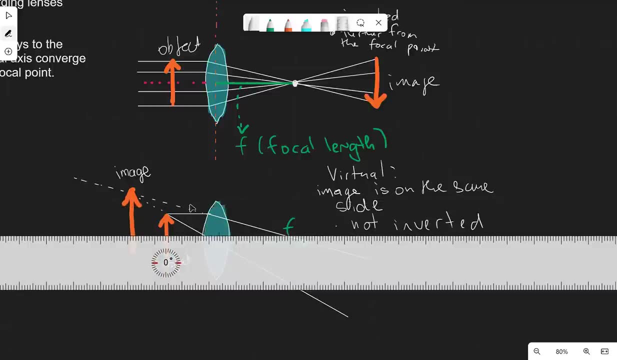 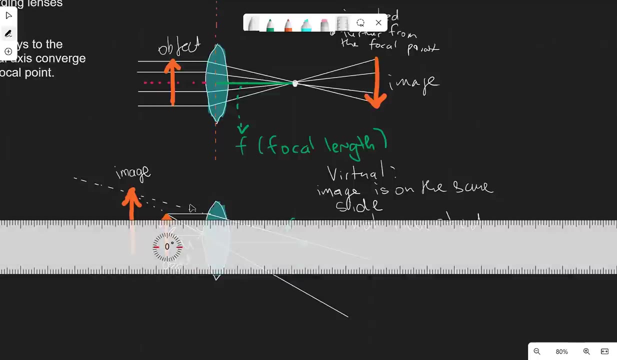 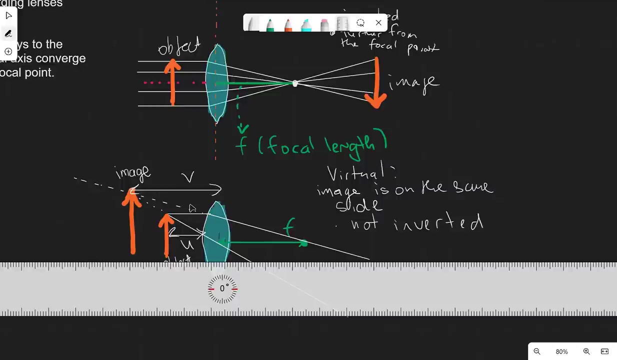 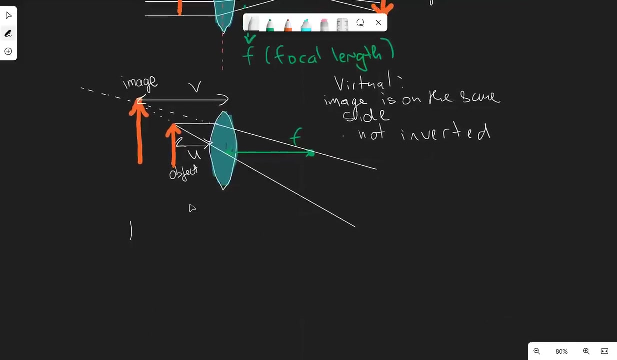 allow us to calculate the positions. So let's say that the distance from the object to the actual lens is known as u and the distance from the image to the lens given by v. The equation that links them together is known as the lens equation and that is given by 1 over f, where f is the focal. 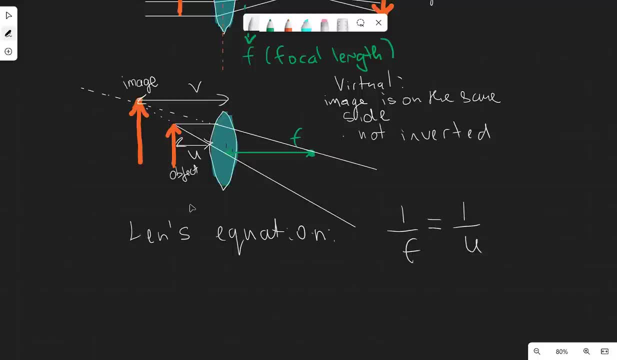 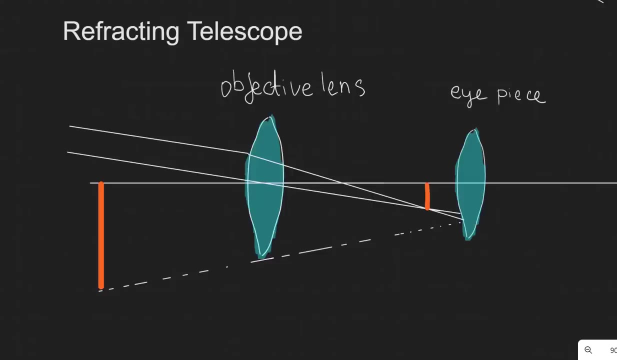 length. So we can do 1 over u, where u is the distance to the object, plus 1 over v, where v is the distance to the image. So refracting telescopes consist of two lenses: One of them is known as the objective and then the other one is known as the eyepiece. 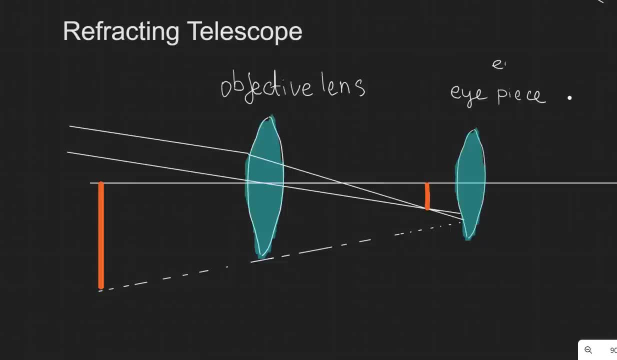 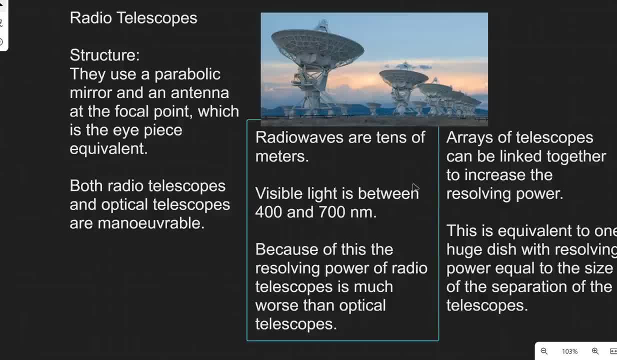 The second lens, the eyepiece over here, is essentially a little magnet which can be anywhere up to tens of meters. They have a very, very similar structure, So they have a parabolic mirror, as you can see in this image over here. 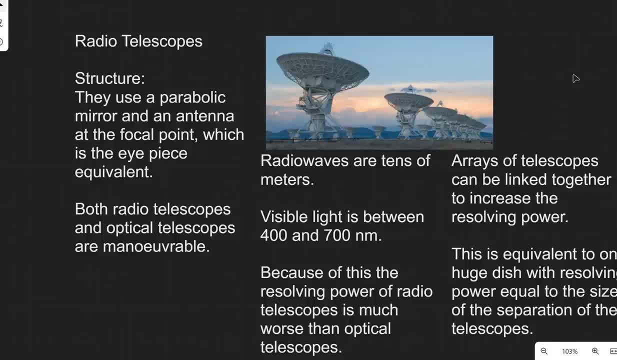 Because it's not visible light. but the data is just analyzed. they're focused at a focal point which is just an antenna. So they're essentially spherical telescopes, but they reflect radio waves. So both of the radio telescopes and the optical telescopes. 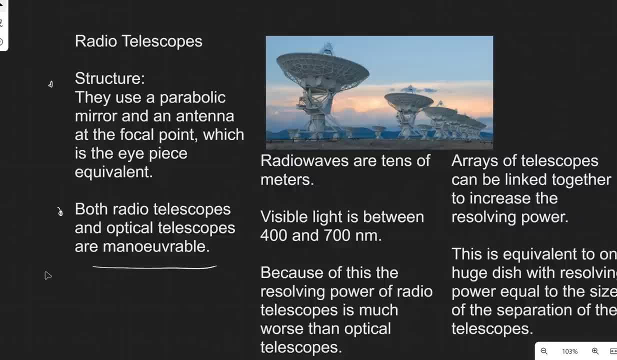 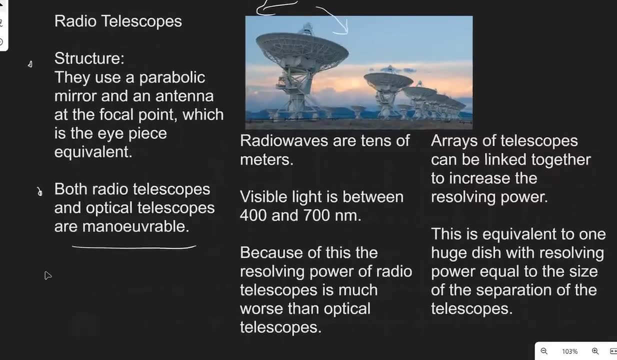 and in fact, all telescopes are maneuverable. What do I mean by that? That means that they can move around these axes to track an object as the Earth is rotating or as the object is moving across the night sky. There is one major difference, though. 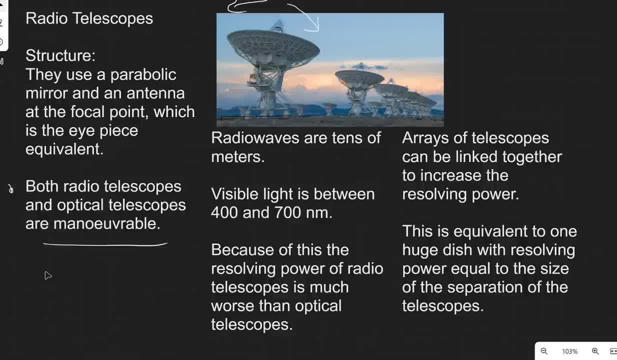 So, as we said, radio waves are anywhere from about a meter, or less than that, all the way up to tens of meters, Whereas, on the other hand, visible light is between 400 to 700 nanometers. So this means that, potentially, the radio waves are over 10 million times longer. 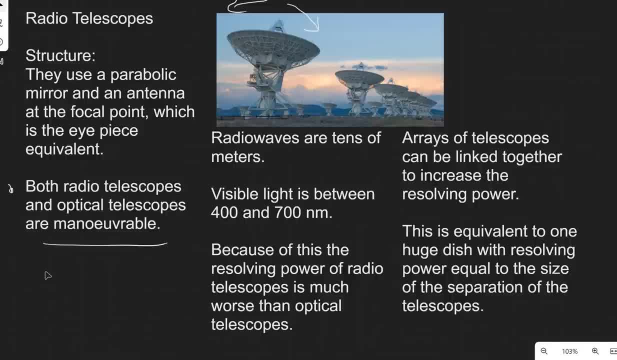 Now, because of that, if you're trying to create an image with a much longer wavelength, the resolving power of radio telescopes, of a single radio telescope, is going to be considerable. It's going to be considerably worse than an optical telescope. 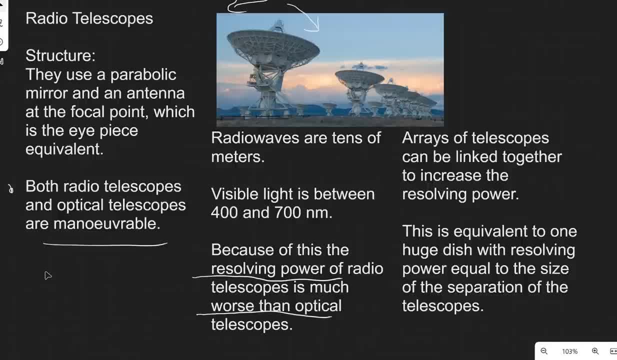 However, there is a catch: You can link multiple arrays of telescopes, sometimes in different locations across the globe, and that will increase their power, equivalent to having one giant telescope with essentially the size of the dish equivalent to the distance between them. 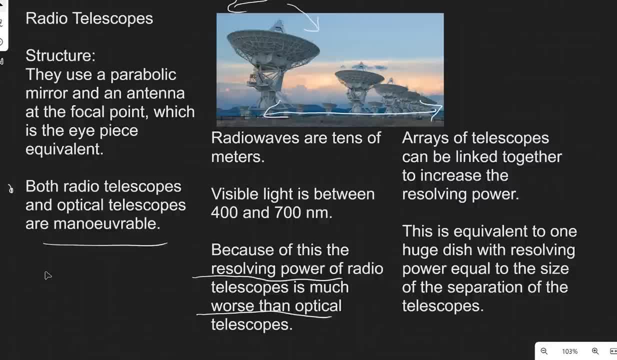 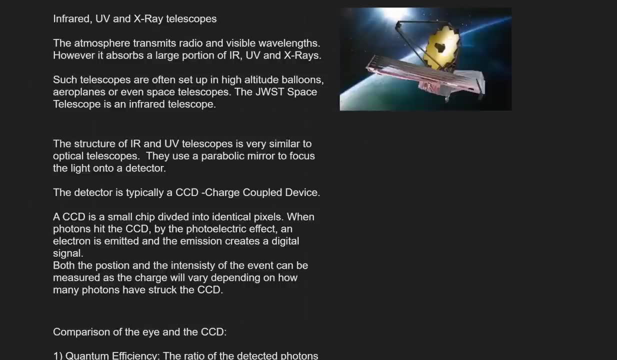 And even if they're in different locations around the world, AI essentially can be used to link them up. This is actually how the first image of a black hole was actually produced, So it is not just radio waves that we can use to build telescopes. 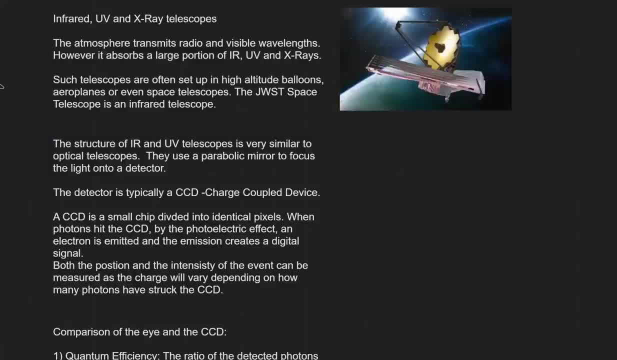 We can also use things such as infrared, things such as UV and X-ray telescopes. The idea, though, is that the atmosphere actually transmits just radio and visible light. The idea, though, is that the atmosphere actually transmits just radio and visible light. 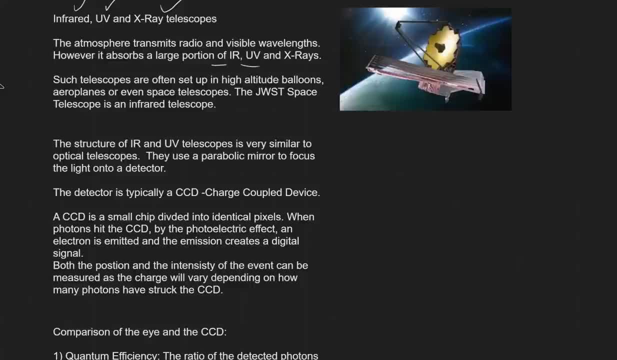 The idea, though, is that the atmosphere actually transmits just radio and visible light, And a very large portion of infrared, UV and X-rays are absorbed by the atmosphere. So if we were to build telescopes that work in the infrared or the UV range, they're often set up in high-altitude balloons, particularly for UV and X-ray radiation, or airplanes or even space telescopes. So for instance, the JWST that has been quite recently a lot on the news, quite rightly so. 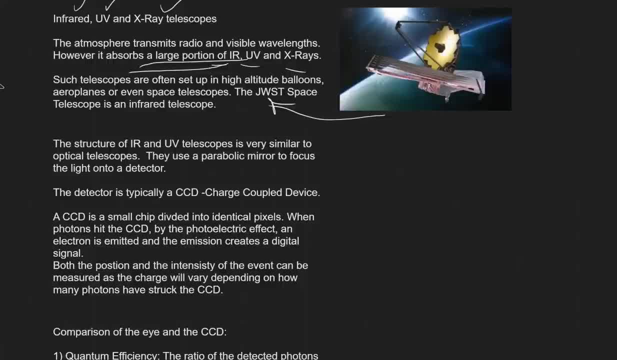 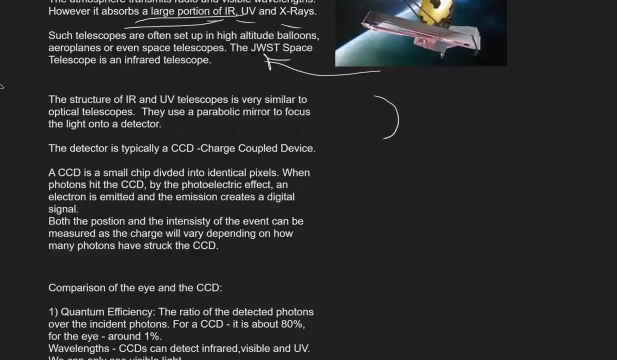 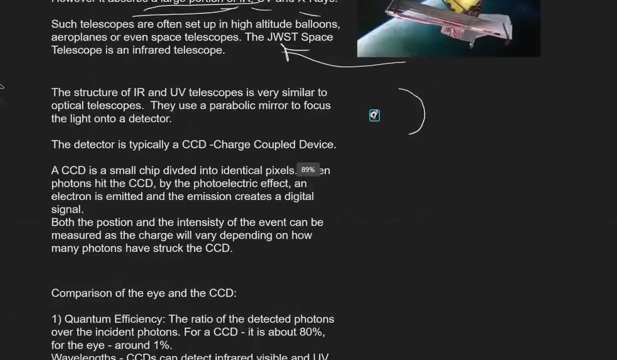 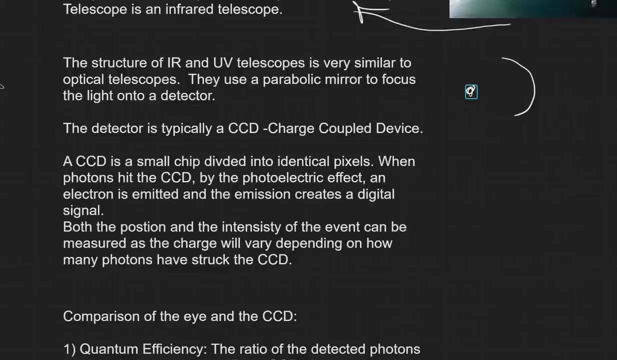 is a space telescope which is an infrared telescope. the infrared and uv telescopes are broadly pretty similar to optical telescopes, so they keep using a parabolic mirror. however, what do they actually focus the light on now? here lies the difference. so they typically use a detector, which is known as as a ccd, which is a charged couple device. so essentially it's a small. 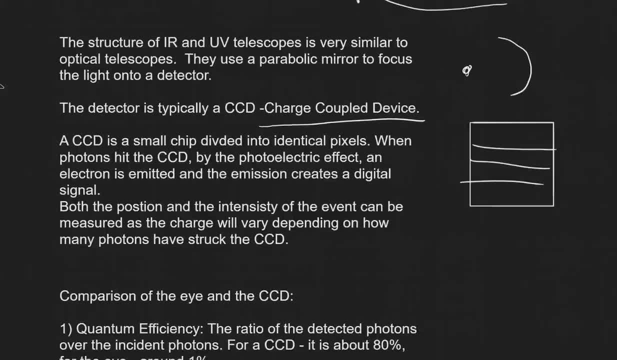 chip that's been divided into millions and millions of individual identical pixels. so if a photon is to strike a pixel, then that would mean that an electron is emitted from there. now, if it's emitted, this would change the charge of this pixel- and this is by the photoelectric effect, by the way- and this will essentially be creating a digital 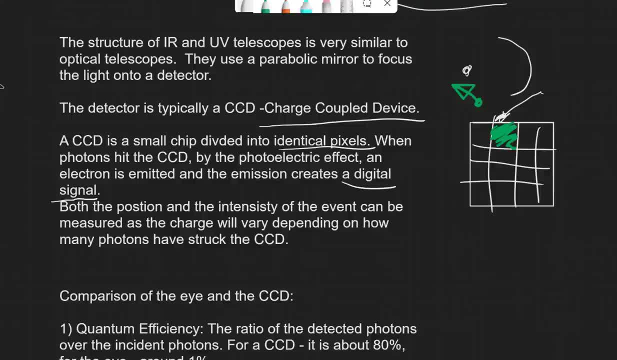 signal from that you can infer both the position and the actual intensity. so, for instance, let's say that we've had a couple of electrons that have flown over from this pixel. you'll have certain intensity. then we will only have a little bit less intense signal if only one of them has. 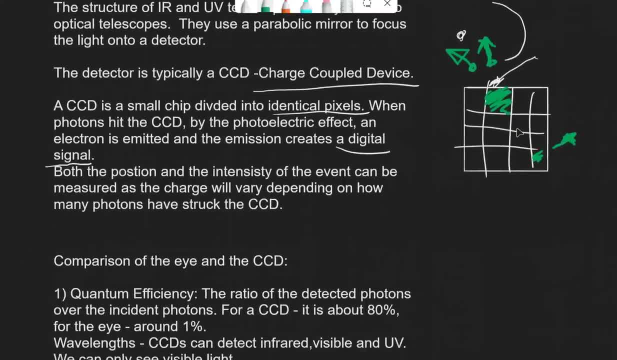 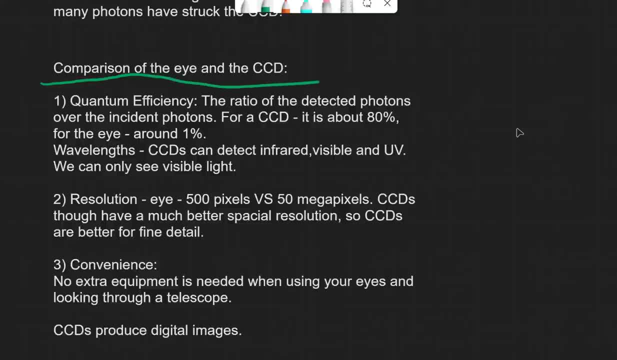 a different signal out of a different pixel. for the exam also, we'll need to be able to make a comparison of the eye and a charged coupled device. the first time that we need to be aware of is quantum efficiencies, so this is simply the ratio of the detected photons over the incident: photons. 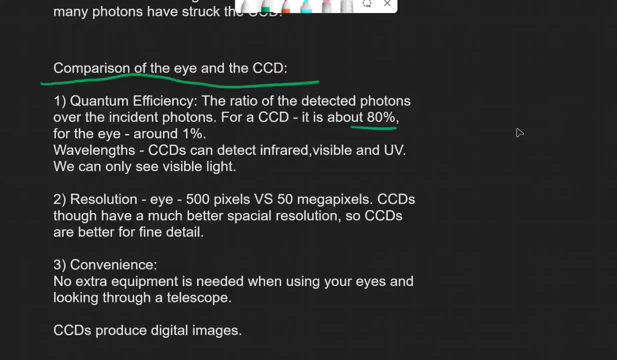 for a ccd this is really high: it's around 80 percent, whereas for the eye it's around one percent. additionally, keep in mind that the ccd scan obviously detect things like infrared visible and uv- not x-rays but infrared visible uv- but we can only detect visible light with our eyes. 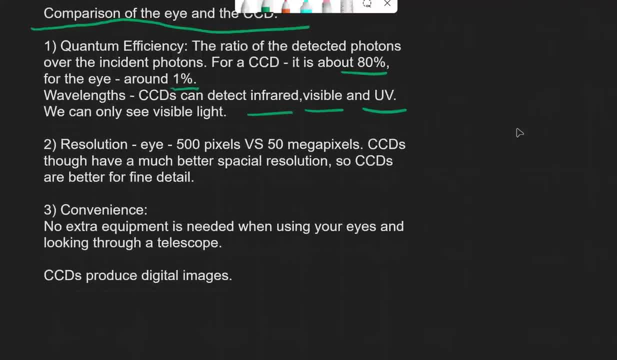 so that's a major limitation. the resolution is an interesting one, so the overall resolution of the eyes around sort of 500 pixels or so versus- probably depending on technology, these things do change every year- around 50 megabits per second. that's kind of an understatement and also at least 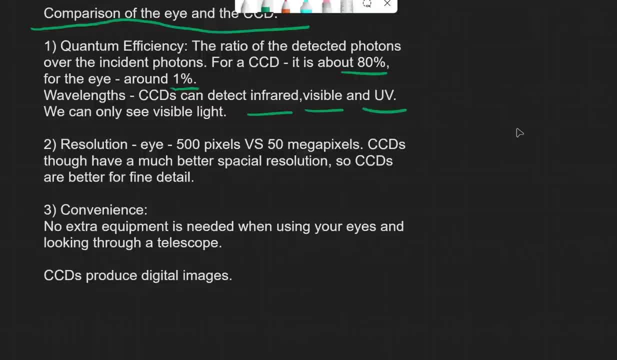 megapixel for a CCD. over the much. they have a much better, what is known as a spatial resolution. that is essentially the resolution required to tell the difference between how far different objects are. and they have a much better one, over ten times better one than the eye. so they're much better for fine. 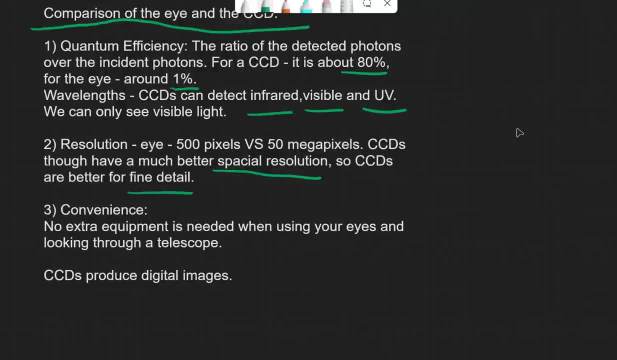 detail. additionally, if you're just looking for the eye lens of an optical telescope, you need no extra equipment when using your eyes. but on the other hand, if you have all the equipment in a UV telescope and things like that, you can produce digital images. additionally, you can look at potentially through 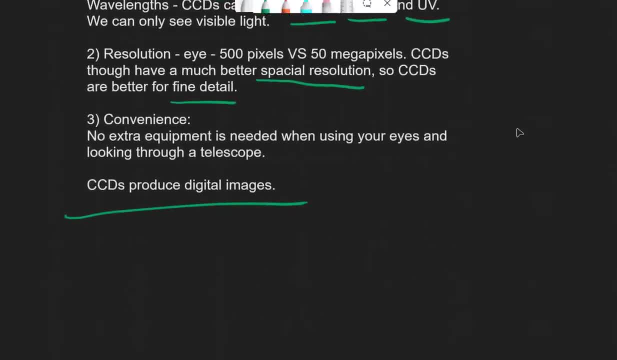 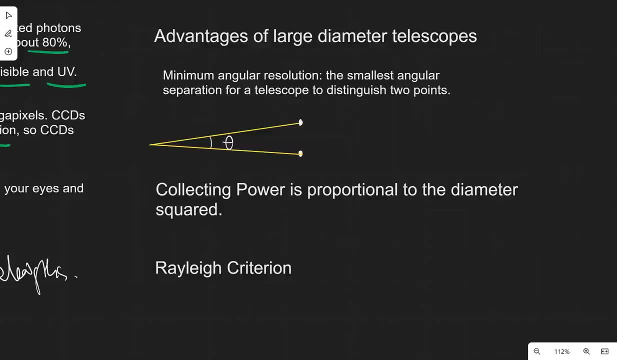 things like nebulae, for instances. so the the next point from the specifications we're going to be revising are the advantages of large diameter telescopes. now, in order to do so, we first need to introduce the concept of the minimum angular resolution. think of it as the smallest angular separation. 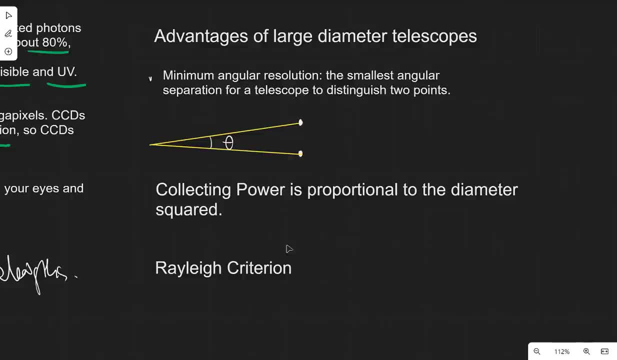 for a telescope to distinguish between two points. so if our telescope is rubbish, those two points are just going to appear as a single point. if we were to get closer and closer and closer, this angle here will become essentially bigger, and we're going to do the same thing for the other side, just in order to have a 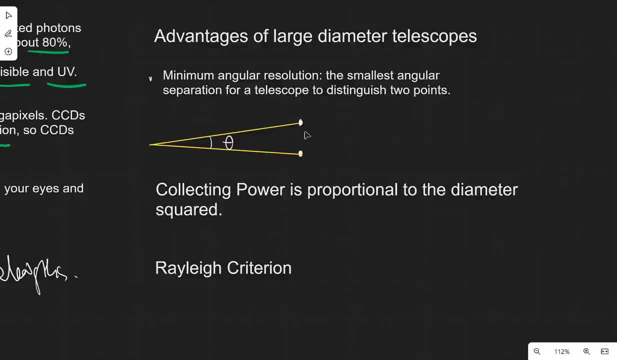 smaller object. so how far apart will this telescope be? in this case, this is, in fact, more than a number of millimeters. the distance between these two points is about a centimeter, but it's not necessarily going to be bigger than a millimeter because of the own dimension, but it will be more closer than a 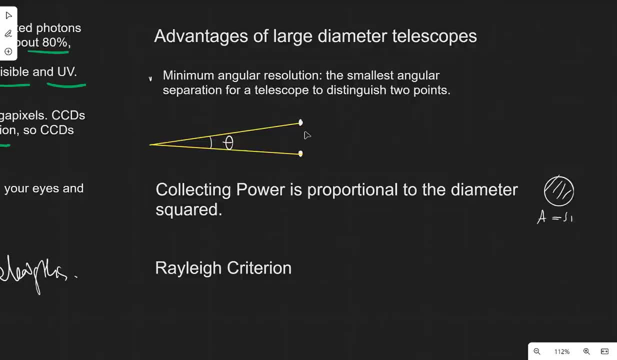 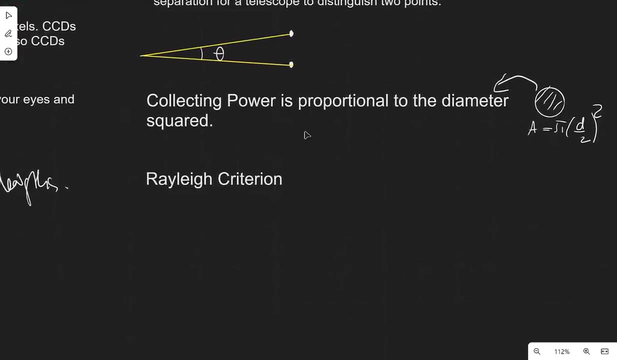 centimeter, and we need to know what the distance between these two points should be, to get close together to the telescope- really comes from What really? what we need to introduce, though, is something which is known as Rayleigh's criteria, and that tells us that the minimum angular resolution- let's call that- 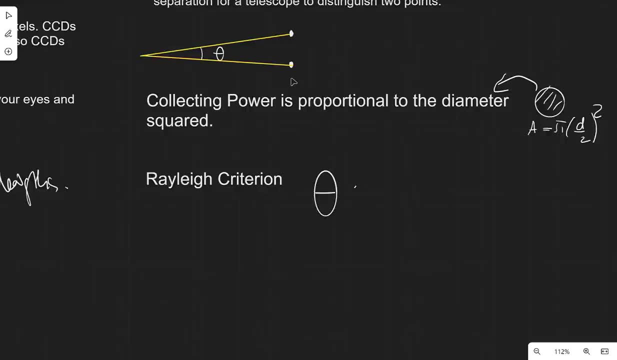 theta, as we have in this angle here, is approximately equal to the wavelength that we're trying to observe divided by the diameter of the aperture that we are using. so the diameter of the aperture is essentially the diameter of our objective lens or of our objective mirror. so 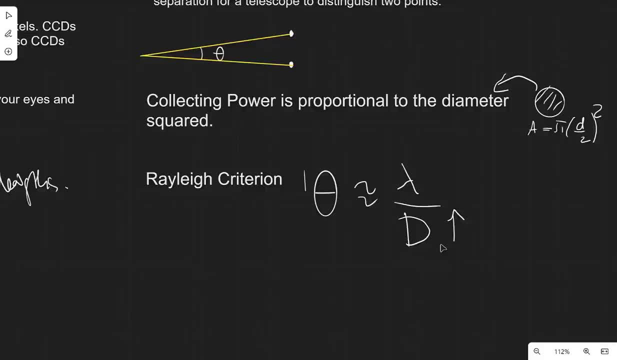 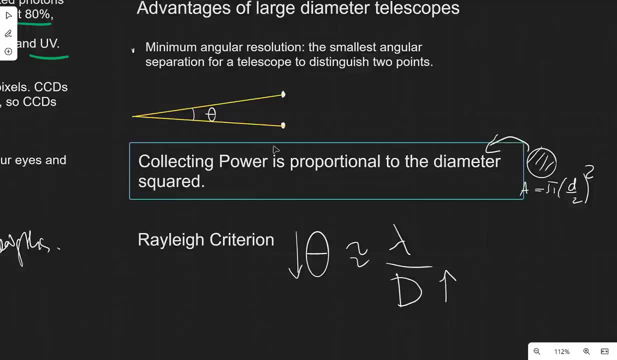 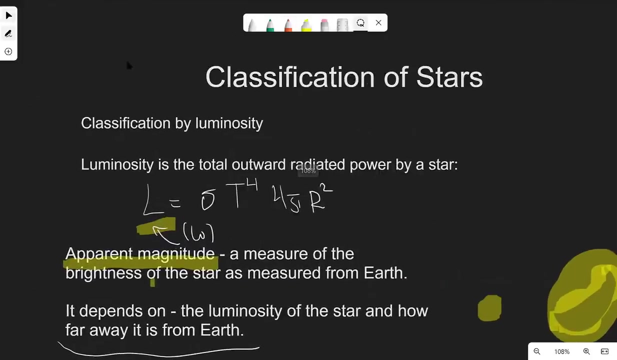 the larger the diameter, the smaller our minimum angular resolution and, in order to have as much detail as possible, we want to keep our minimum angular angular resolution as small as possible. And now let's talk about the classification of stars. We're going to start off by classification by luminosity, which essentially is a measure of 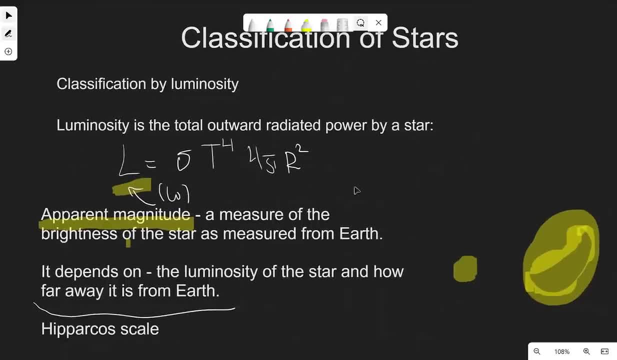 the brightness. Well, let's introduce the term luminosity, even though it appears a little bit later when we do Stefan's law. Well, luminosity is the total outward power radiated by a star. It's given by this equation, which we're going to look at in our next chapter. 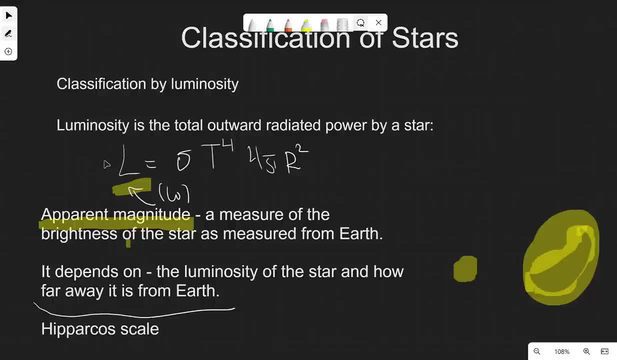 but in general it is just power. it's what astronomers call power. it depends on things like a constant and then multiplying by the temperature raised to a power of four, and then the surface area In general, the brighter the star is, either the temperature is much higher or its radius is much higher. It's just measured in watts. 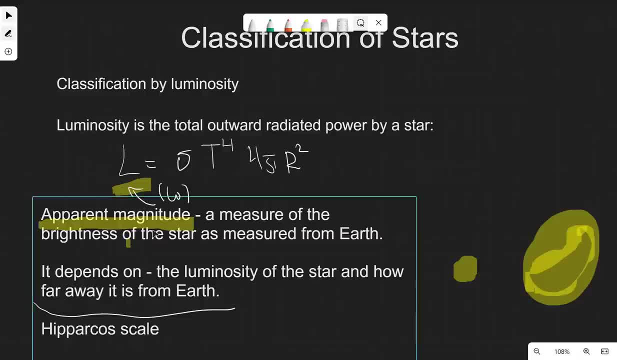 Okay, well, one way of classifying stars is by apparent magnitude. Now, this is a measure of the brightness of the star as seen from the earth, which is really, really important. It depends on the luminosity of the star, its power and how far away it is from the earth. 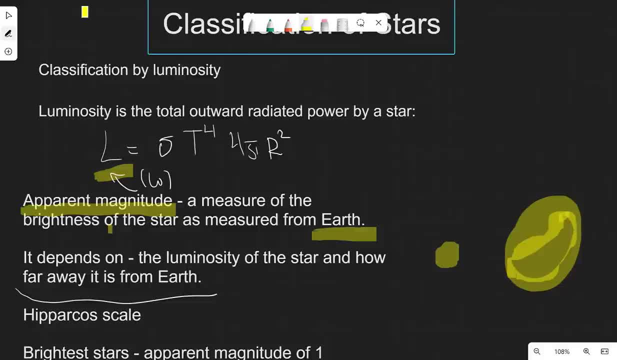 For instance, if i had kind of a small star, this here will have a relatively low luminosity and this large star will have a higher luminosity. However, if the small star was much closer to the earth, then it will appear a lot brighter. The first person to come up with a form of classifying 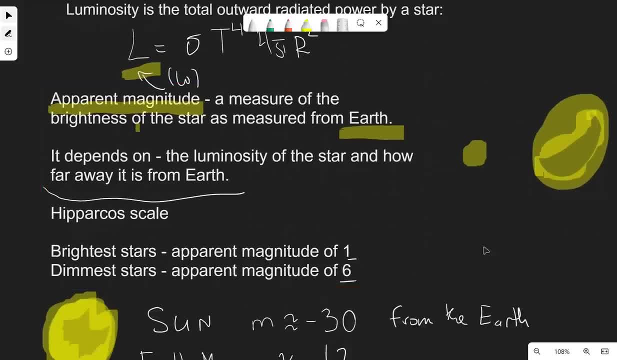 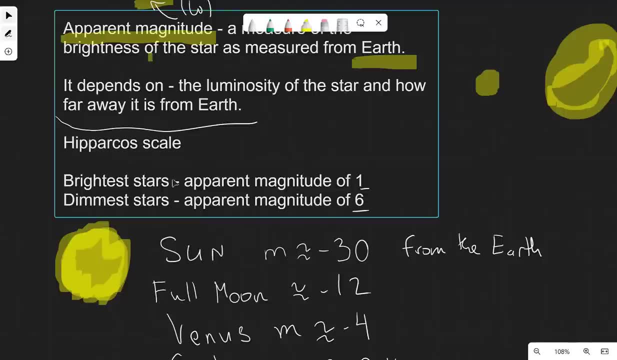 star was a chap called Hippoparchus, who lived in ancient Greece, and he came up with a scale: The brightest stars were given an apparent magnitude of one, and then the dimmest stars were given an apparent magnitude of six. These days, we've replaced 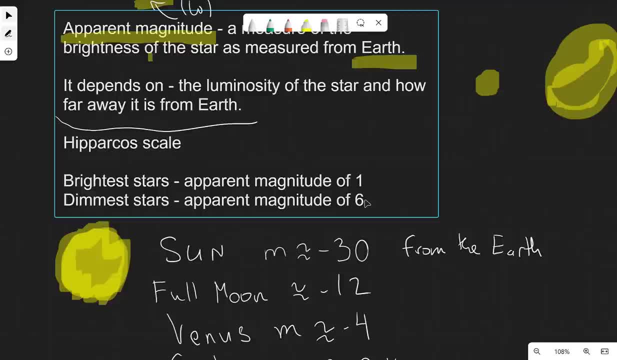 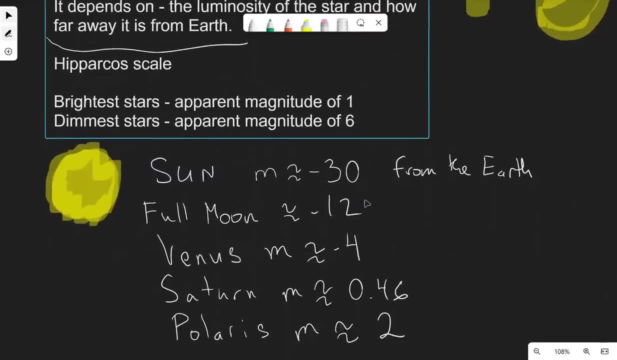 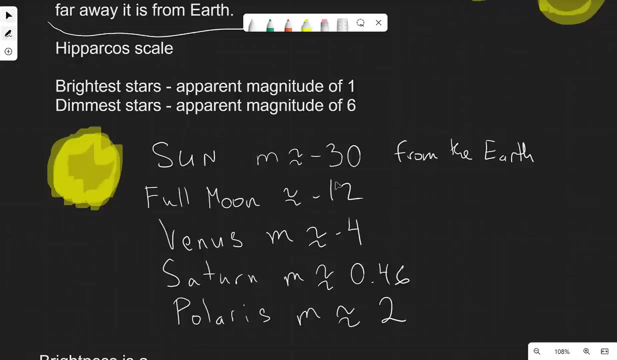 this with a far more sophisticated logarithmic scale and, in general, the lower the number or the more negative the number, the brighter it is, And all these values below are taken or measured from the earth. on average, For instance, the sun has an apparent magnitude of around minus 30.. A full moon. 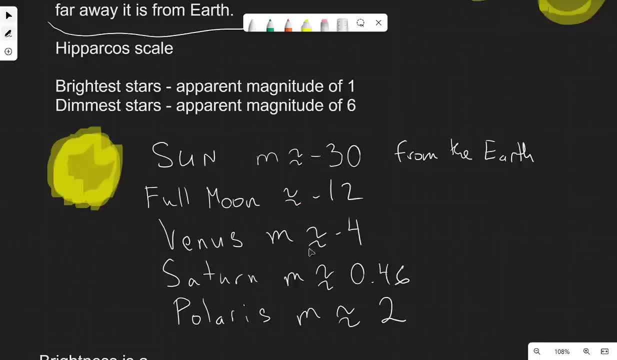 will be somewhere around minus 12.. Venus will be around minus 4.. Saturn around 0.46 on average. Polaris, the north star, around 2.. So you can see that the really negative numbers are very, very bright, and then the positive, bigger numbers are very, very dim. Well, remember though. 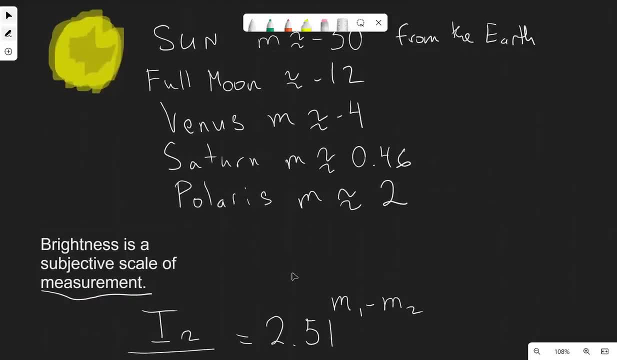 brightness is a subjective scale of measurement, and this is really, really important. It depends on things like the distance, and you can have two measurements which would know, which may not necessarily be the same. For instance, if Venus is a little bit closer to to to the earth, it will. 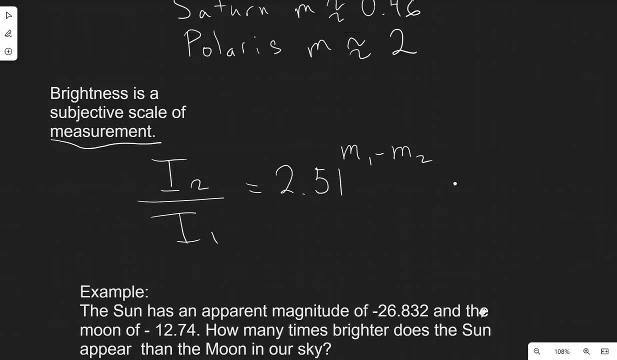 appear brighter. We also need to know about this equation right over here which gives us the ratio of two intensities as measured from the earth, and that is equal to 2.51. and this ratio here, or this difference here, M1, take away M2 is the difference in apparent magnitude. Well, let me give you an. 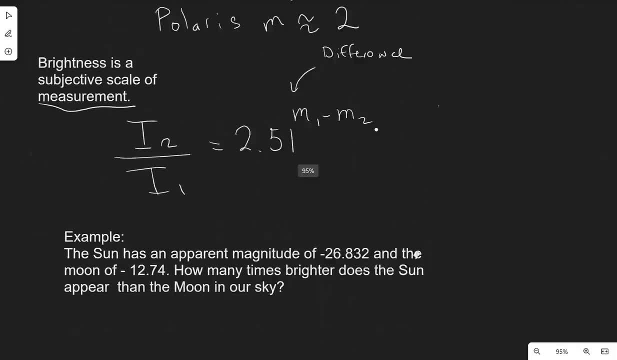 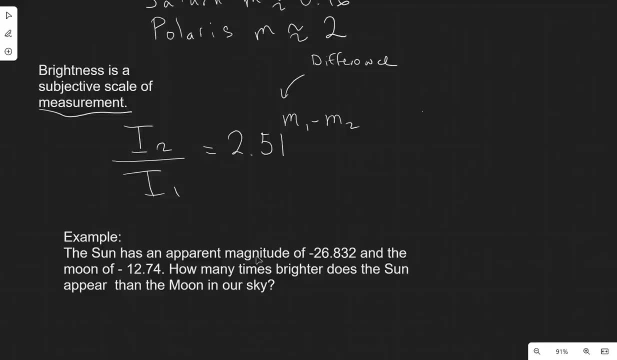 example for this. We have the sun, which has an apparent magnitude of minus 2.6832, then the moon- oh, what's happening here? let's get rid of that- the moon, which has an apparent magnitude of minus 12.74.. How many times brighter does the sun appear than the moon? 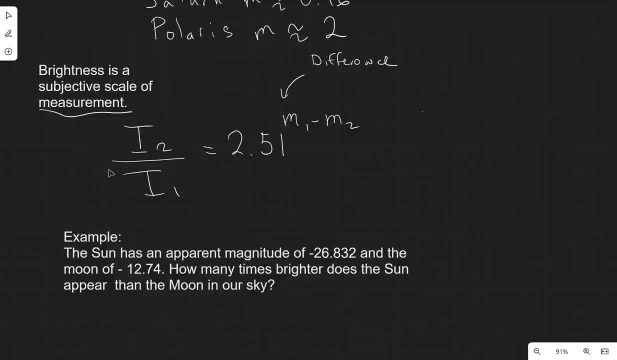 in our sky. Well, because I'm going to be finding out how many times is the sun brighter than the moon. in this case, I'm just going to take the index 2 to relate to the the sun. so I2 will be the intensity of the sun and I1 will be the intensity of the moon. Well then, this equation: 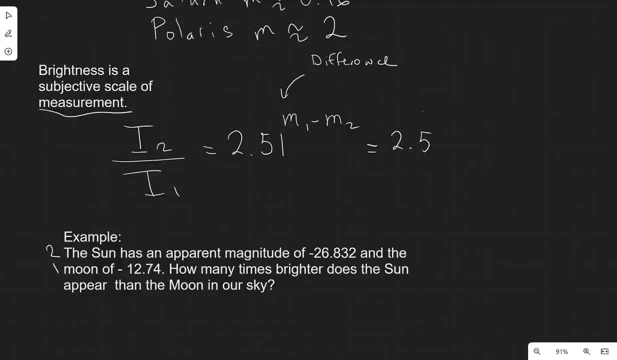 will tell us that this ratio will be equal to 2.51, and this ratio will be equal to 2.51.. Raised to the apparent magnitude of the moon, which is minus 12.74. so minus 12.74, then we're going to take away a negative number, which is the apparent magnitude. 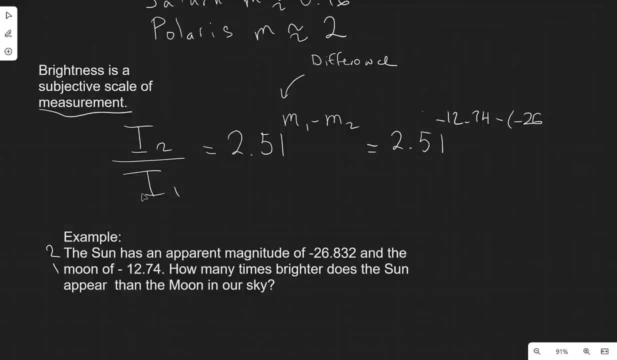 of the sun. so that'll be minus 26.832, which is equal to 2.51, raised to the power of minus 12.74. plus 26.832, which is equal to 2.51, raise to the power of plus 14.09, and this will be a very large number. so if in our calculator, 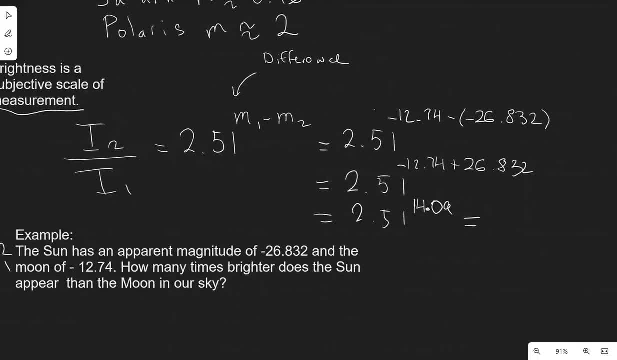 we do 2.51 raise to this power, we're going to get a number well over 400 000, so vamos ir bem mais de 400 000es. então em mogamos ver um número de 2.51에 y bienvingado owners das linhas que producemos um número de 2.51 e cobrando um número de 14.09.. 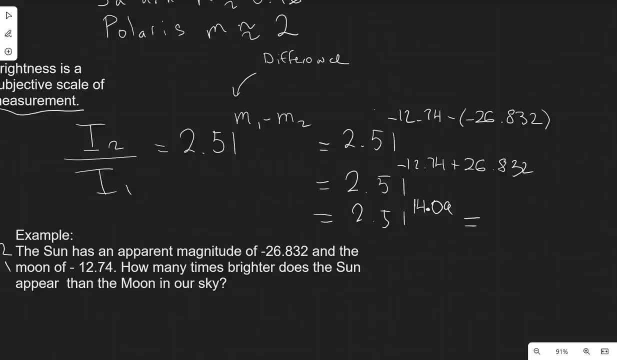 400,000, so around 432,500, up to around four significant figures. so the Sun is this many times brighter. the relative intensity of the Sun is 432,500 plus times brighter than the moon in our sky. now for the next portion of the spec. 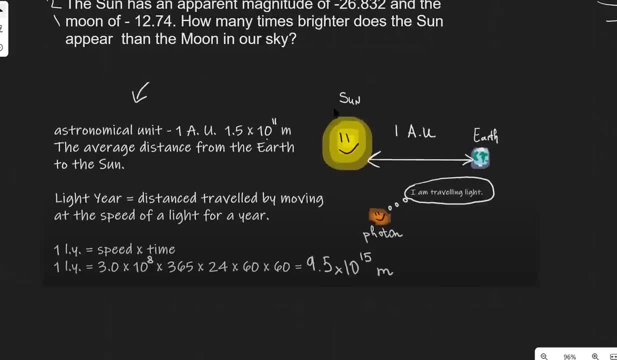 we need to first of all define some units that we're going to be using quite a lot. so these here are units. first of all, we have the Astronomical unit which you probably come across at some point. it's known as one au and that's. 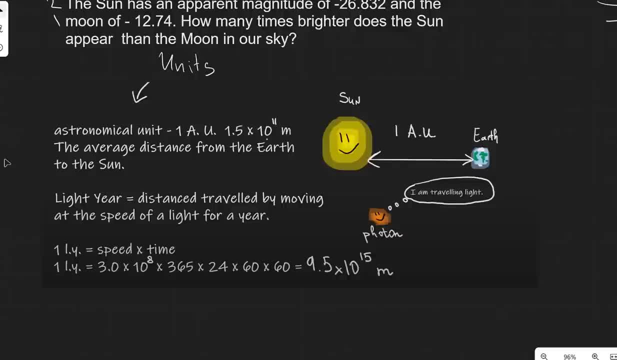 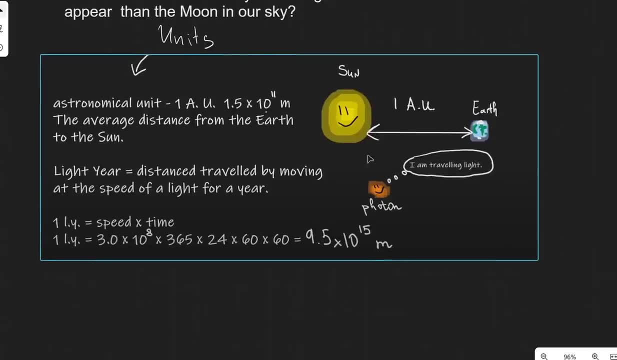 around one point five times 10 to the 11 meters. it's defined as the average distance from the earth. here's the earth to the Sun. because one meter as well is not useful, very useful as a measuring unit and babbling. but there is a mention here something called star pressure. this is basically 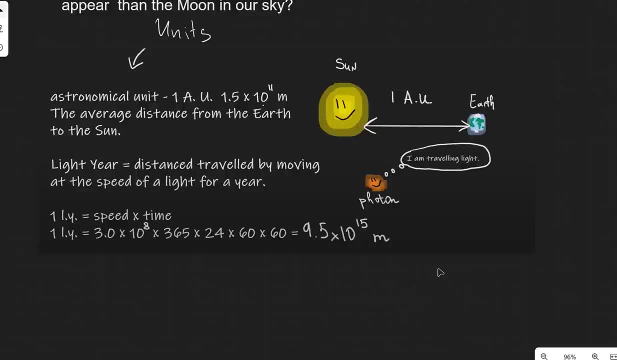 as a meter stick across the universe. the universe is far bigger than that. we're also going to need to define a light year. that is the distance traveled by by moving at the speed of light for one year. let's calculate how much that is, because the speed of light is constant. 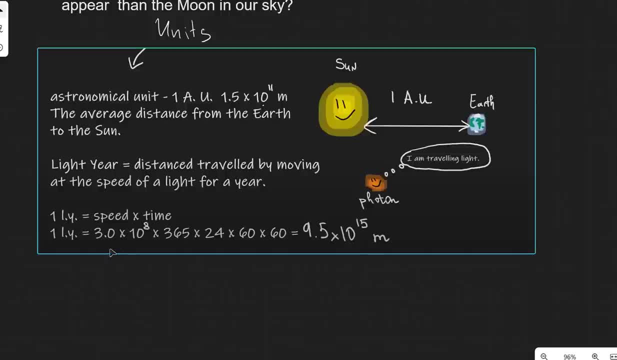 one light here is going to be equal to speed multiplied by time, which is going to be 3 times 10 to the 8 times 365 times 24 days. each of them has um 16 times 24 hours times 60 minutes. multiply by 60 seconds and this will give us a grand total of 9.5 times 10 to the power of 15. 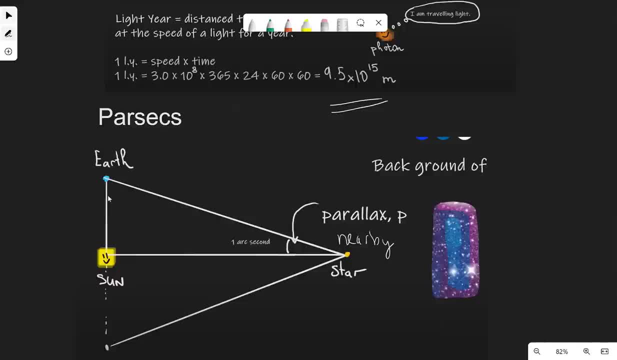 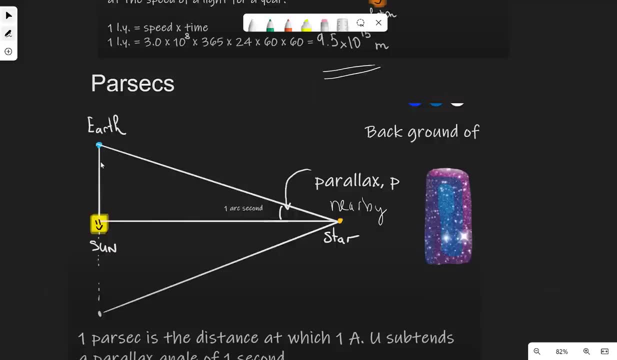 meters, and this is one light here. so the next thing that we're going to be discussing is the unit of distance, which is known as parsec, and that is very much connected with the parallax angle. now let's start off with the basics. imagine that we have the earth across here. we have a 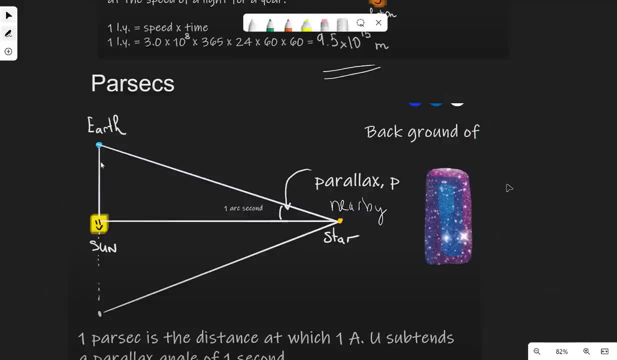 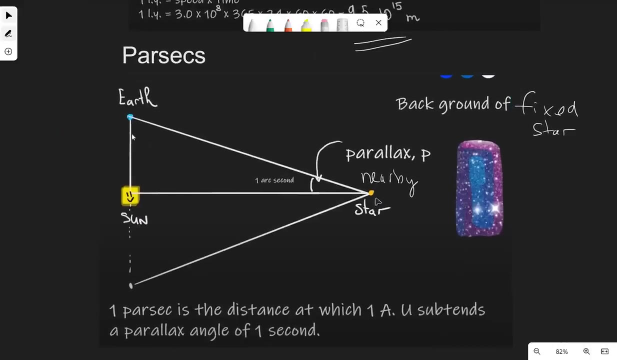 nearby star and we have a background of fixed stars. now they're so far away that their relative position in the background does not really change as the earth is moving around the sun. okay, so let's say that we want to measure the distance to this star if the earth moves across the sun in six months. 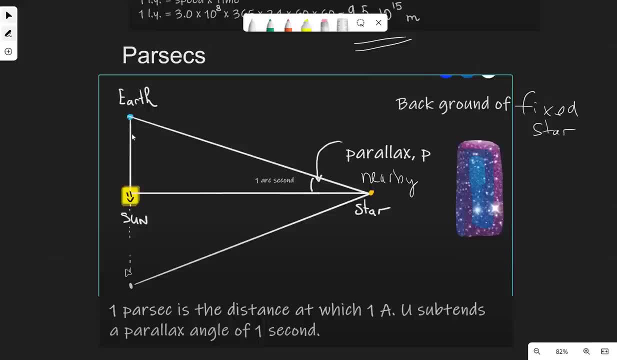 time. then the earth would have gone across half of its orbit and will be able to go to this side. now the position of the star in the night sky would have changed by this angle. here, half of that angle is defined as the parallax angle, and that is very, very small normally. 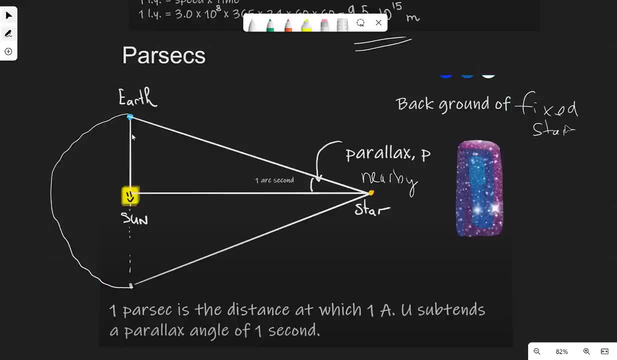 it's a few, sometimes even less than an arc second, and one arc second is defined as one over 3600th of a degree. so it's a very, very tiny number. so we know what the distance for between the earth and the sun is. we've just mentioned that it's one astronomical unit. then if we know this and 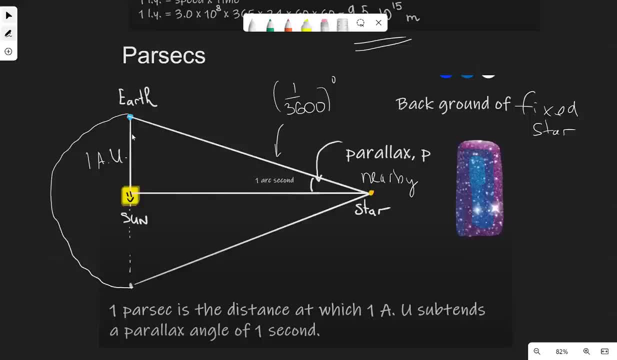 we can calculate this in in meters, then we can use some simple trigonometry. if we just measure the parallax- parallax angle with telescope, this is the exact technique that is used to estimate the distance to nearby stars. now the parsec is this distance across here, one parsec. 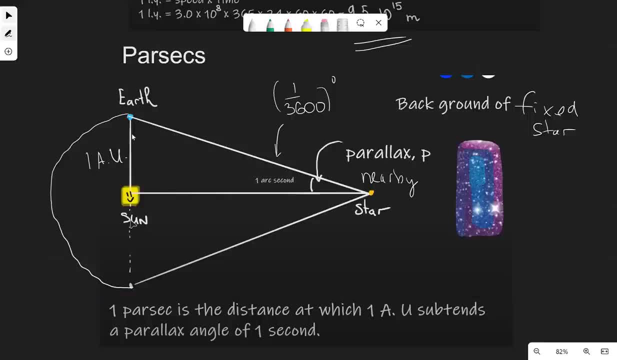 is defined as the distance at which one astronomical unit subtends a parallax angle of one arc second. oops, let's just add one arc second in this definition here. so this means that if this angle here is one arc second, if this here is one astronomical unit, then this distance here. 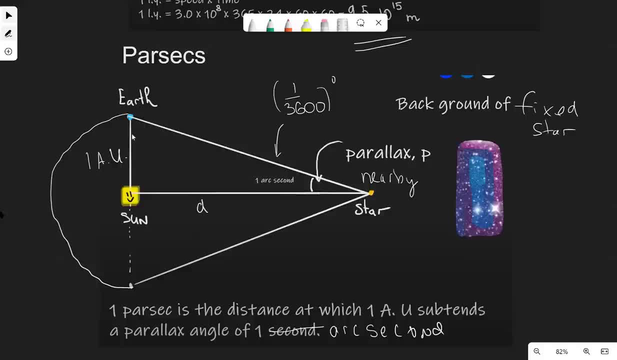 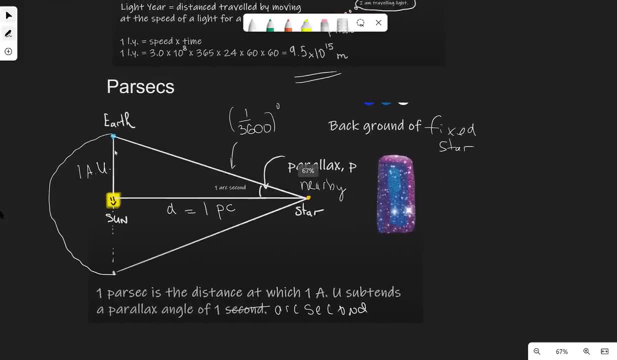 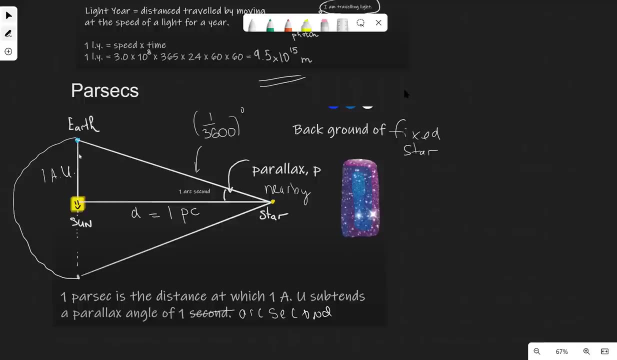 typically given the symbol d will be equal to one parsec, one p c. okay, well, let's estimate the or let's calculate the value of one parsec using some simple trigonometry. so i'm going to use the fact that the tangent of one arc second is going to be equal to. 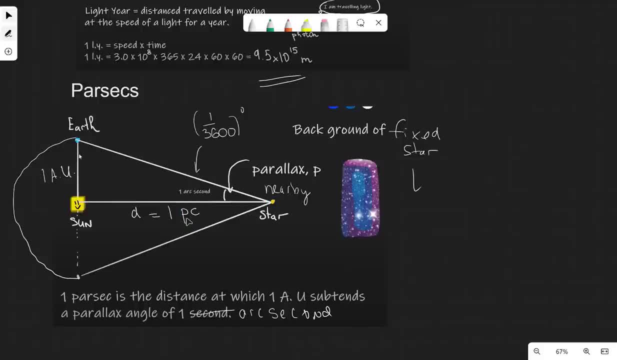 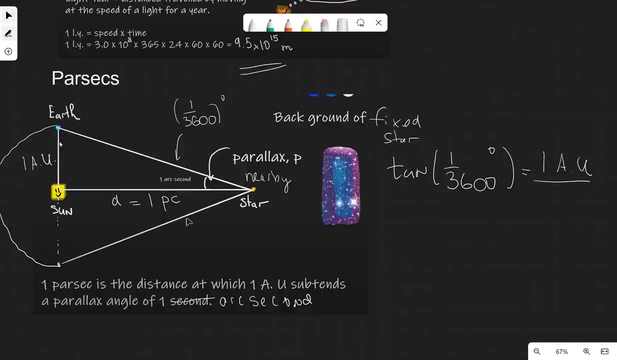 its opposite, divided by the adjacent, so tan of one over three, six zero, zero degrees will be equal to the opposite, which is just one astronomical unit, one a, u, and then we're going to be dividing that by the distance in parsecs. well, remember 1a, u, we've already calculated that value, so we can. 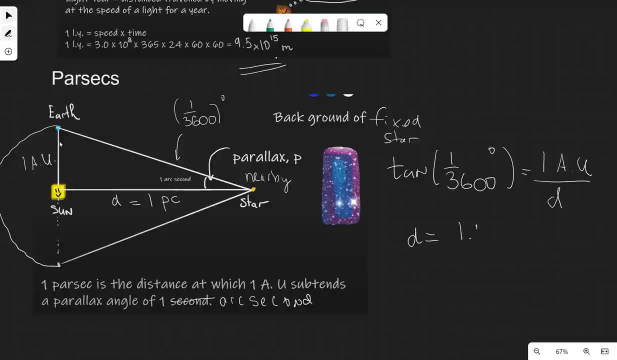 do it in one metric, so that is equal to 1a? u. now let's convert that to meters, which was 1.5 times 10 to the power of 11.. then we're going to be dividing that by the tangent of one arc. second, 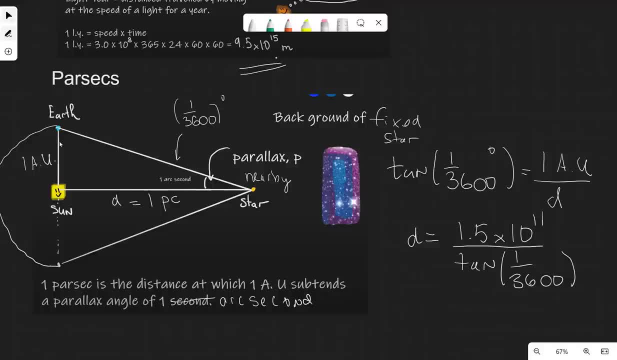 which in degrees is 1 over 3600 and then up to two significant figures. we're going to get that this is about equal to around 3.1, let's call it. i think 3.8 is the accepted value times 10 to the power of. 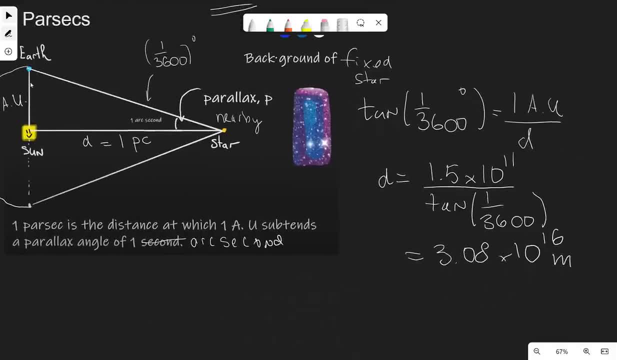 16 meters, and this here is equal to the amount of meters in a parsec. I have a very, very detailed video about this and I'm going to link this in if you want a little bit more detail on this topic. As I said, there's a problem with absolute. 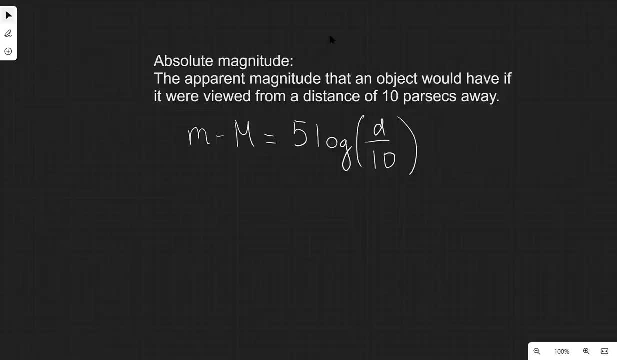 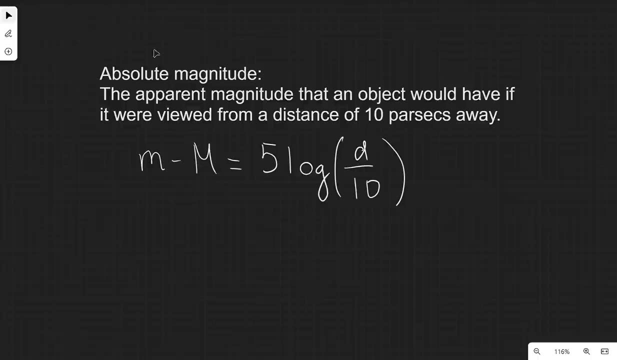 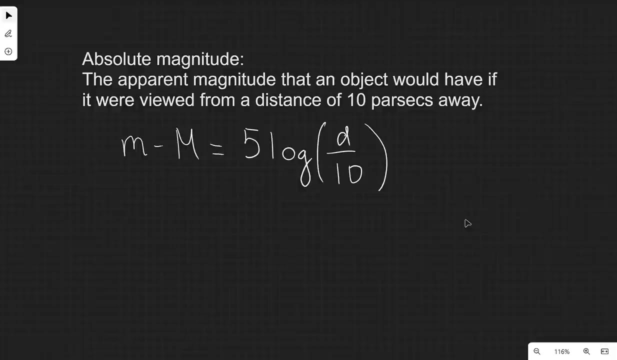 magnitude, and that is that it depends on the distance. So in order to really understand how bright a star is if it were a fixed distance away, we need the absolute magnitude. So this is defined as the apparent magnitude that an object would have if it were viewed from a distance of 10 parsecs away. And we can 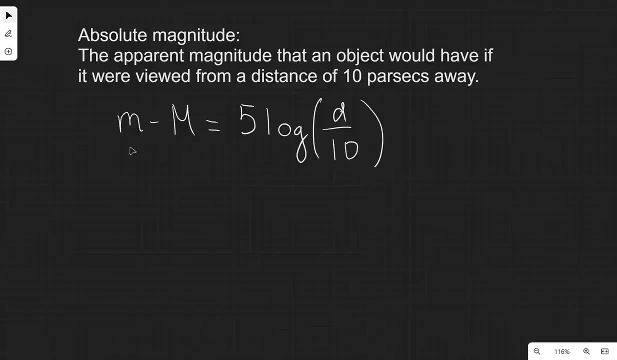 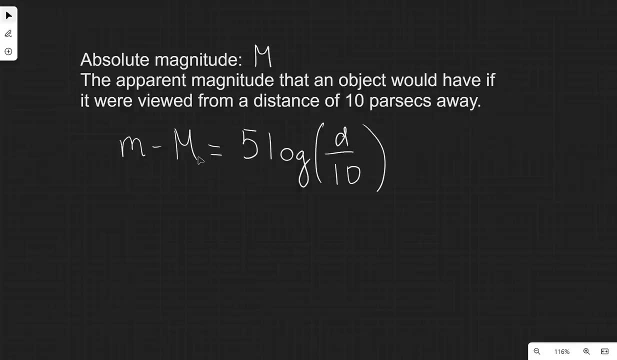 find that using this formula over here, where M take away capital M. So the absolute magnitude, by the way, is typically given the symbol capital M, and that's just this. The apparent magnitude is this, and that is a logarithmic equation- is equal to 5 log the distance divided by 10.. Now, important that this distance has to be. 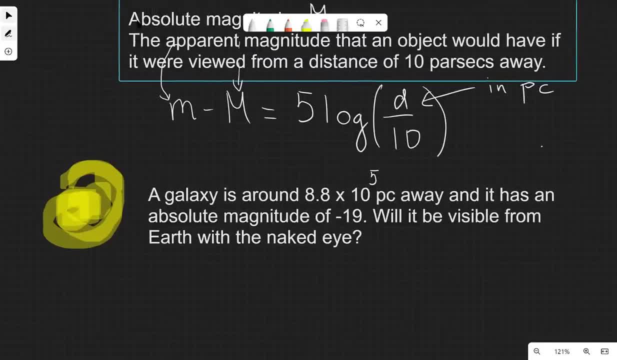 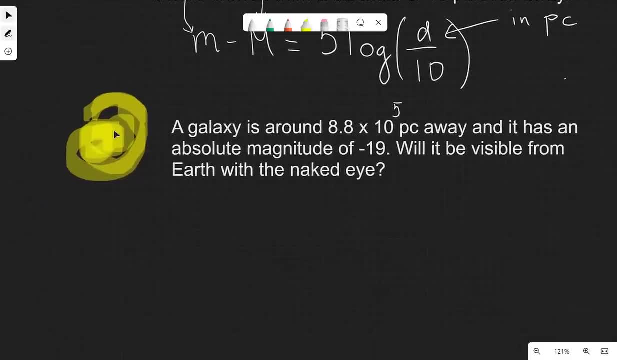 in parsecs. Well, let's apply this equation here to a little example, to make sure that we really understand this. We have a galaxy there. it is of around 8.8 times 10 to the power of 5 parsecs away, and it has an absolute 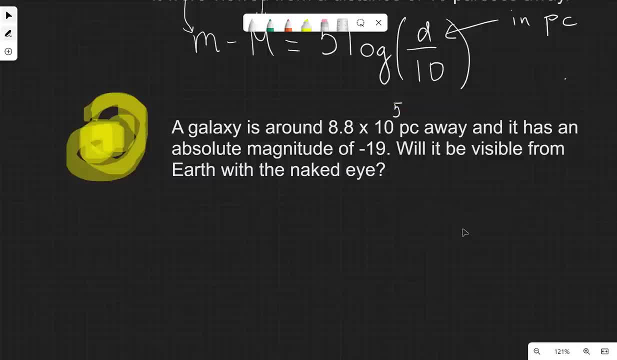 magnitude of 10 to the power of 5 parsecs away, and it has an absolute magnitude of 10 to the power of 5 parsecs away, and it has an absolute magnitude of negative 19.. Now will it be visible from Earth with the naked eye? Now my plan. 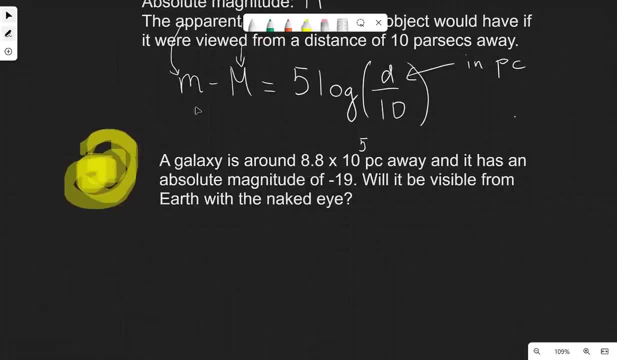 here is to find its apparent magnitude, then how, and then see how it compares on the scale. So I'm gonna use this equation here. I'm gonna just rearrange for M. I'm gonna find that M will be equal to 5, log D over 10, and then plus the absolute. 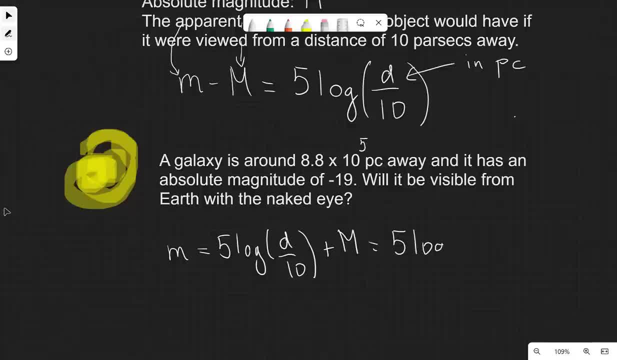 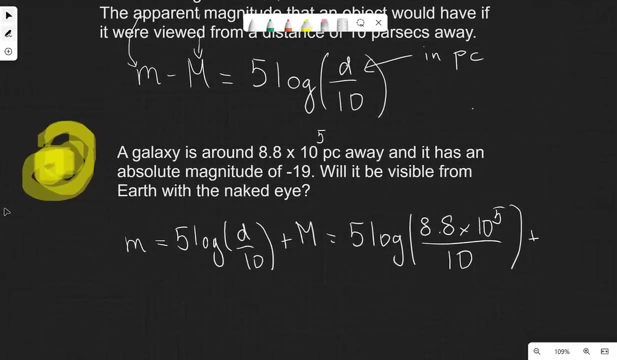 magnitude will be equal to 5 log, and now the distance is 8.8 times 10 to the power of 5. then I'm going to be dividing that by 10, and then to that we must add the absolute magnitude m, which is minus 19, like. 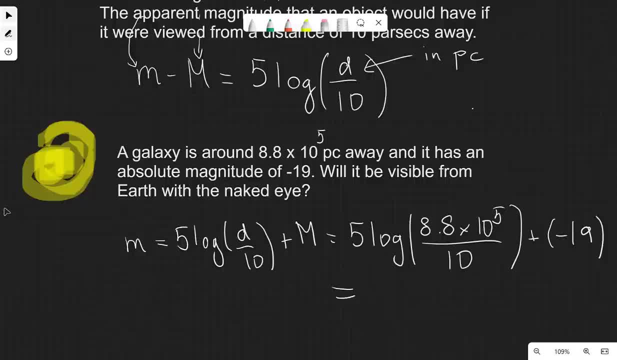 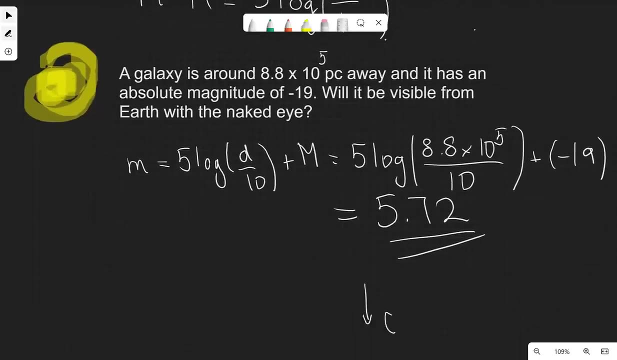 so for to put this into a calculator, we're going to get an answer of around 5.72. well, if you guys remember the Hipparchus scale, that went up to around 6 at the lowest end. so we can assume that things that are as that are, between 1 and 6 and lower, will be definitely 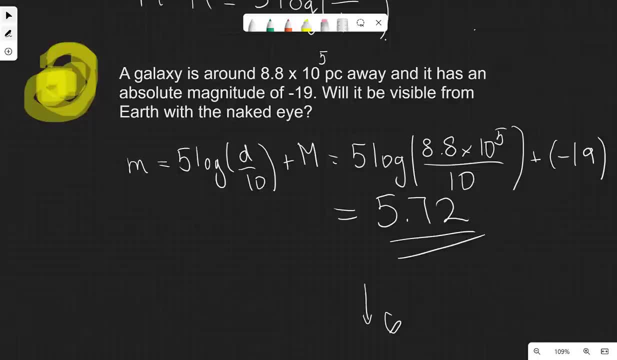 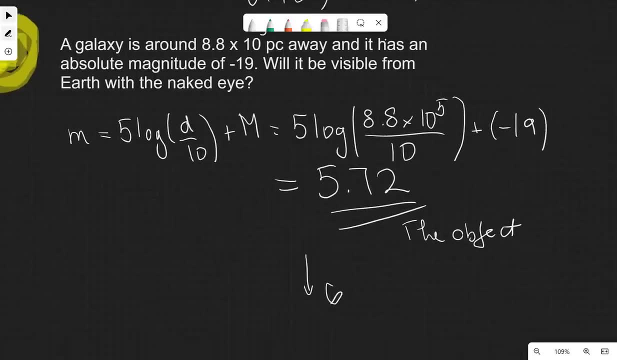 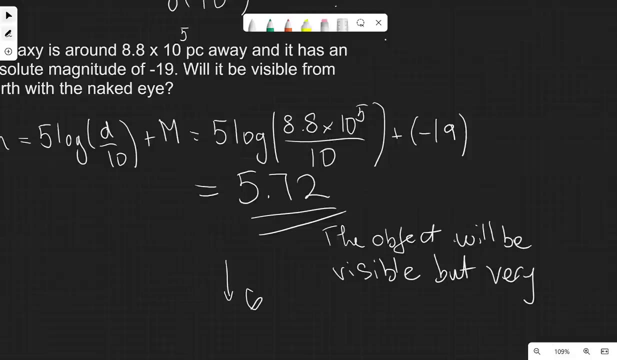 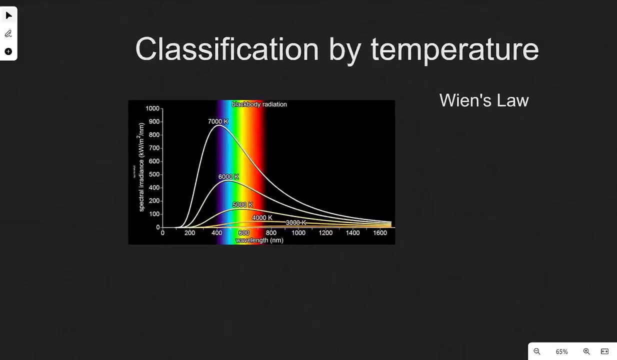 visible. So if it's 5.72, we can say that the object, whatever it is- galaxy, asteroid, supernova, it could be a whole bunch of things. the object will be visible, but very dim. and now let's have a look at classification by temperature. First of all, we need to recognize the blackbody radiation curve. 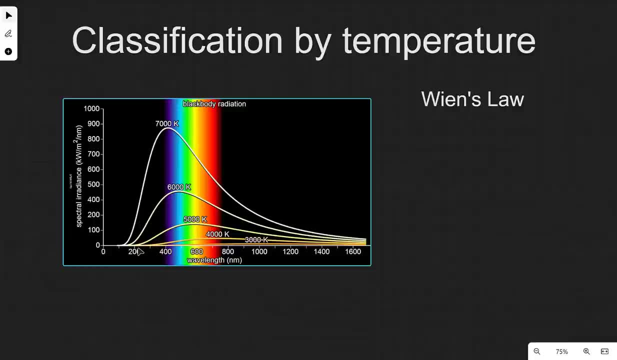 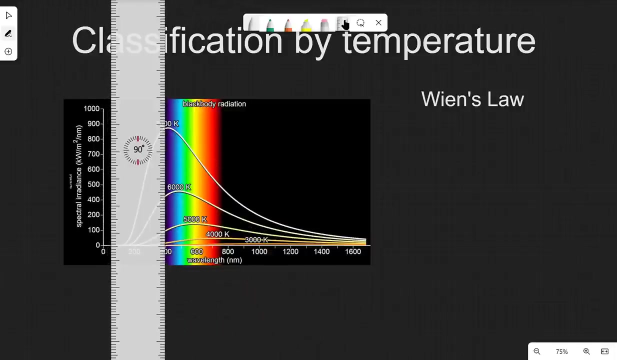 and that is illustrated in this figure right here. notice something interesting: if the temperature is very, very hot- so this here is the temperature of a body of around 7 000 kelvin- then it will emit a relatively low wavelength. we can actually demonstrate that with my digital ruler, so we can see that the wavelength for 7 000 is around here. 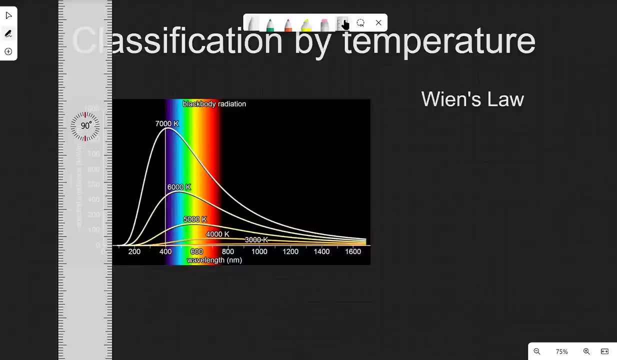 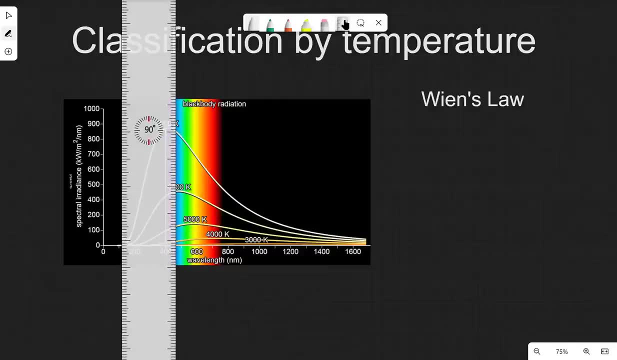 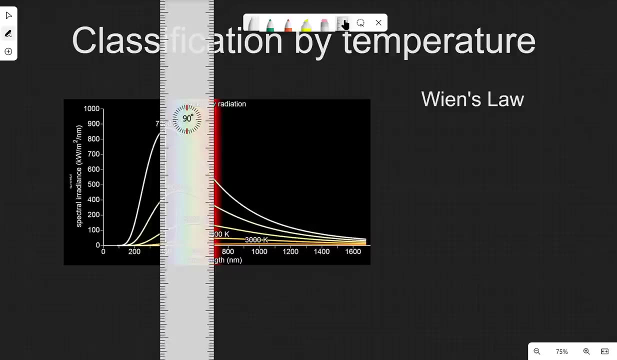 well, the predominant wavelength, the one which is most likely to be emitting for a body at 6 000 kelvin, well, the wavelength will be a little bit bigger. for the one at 5 000, it will be a little bit bigger still. in general, the lower the temperature, the bigger the wavelength, it seems. 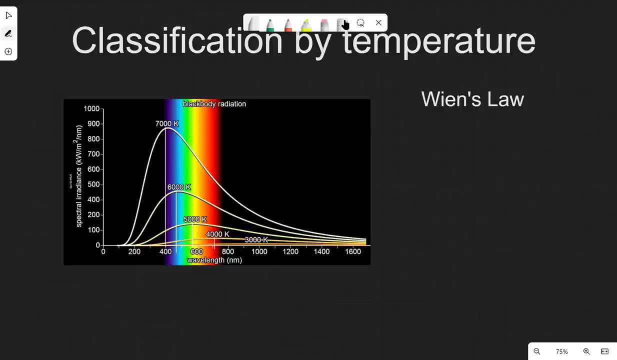 so this will be an inversely proportional relationship. so the most dominant wavelength is the one which is most likely to be emitting for a body at 6 000 kelvin. now, the peak wavelength is often written as lambda max, and this will be proportional to a constant. i'm going to call it k for now, divided by the temperature, another way of writing. 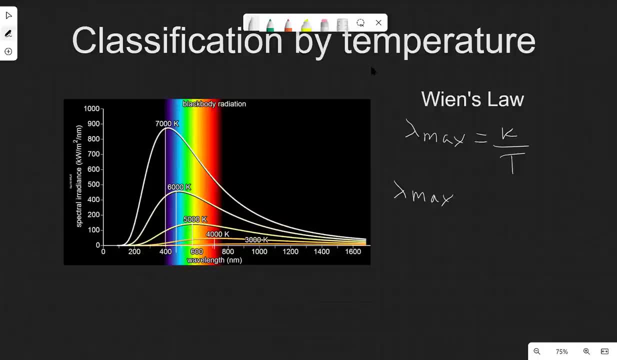 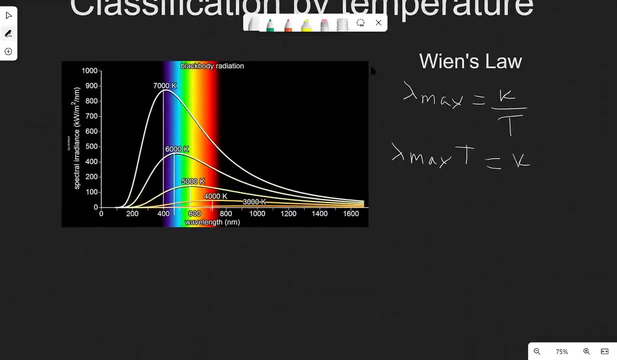 this law is that lambda max times the temperature is equal to the constant k. now this value k is equal to the constant k, so the peak wavelength is often written as lambda max, and this will be OK. um is actually. let's write this down as lambda max times the temperature. 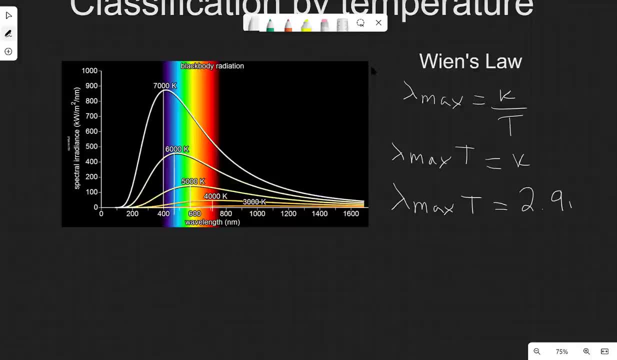 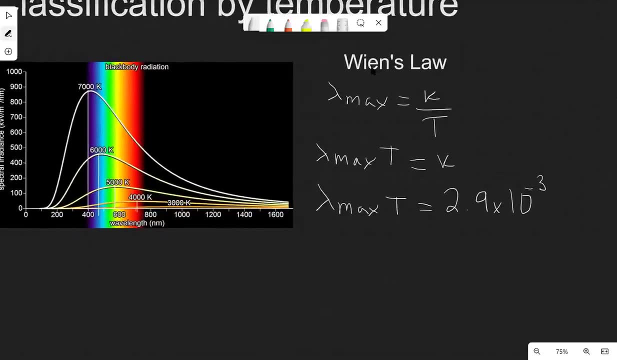 is equal to the value of the constant, is 2.9 multiplied by 10, to the power of minus three. what do you think the unit of this will be? well, its wavelength measured in meters, multiplied by temperature, and this has to be measured in kelvin, otherwise it will not work. so it will be meters. 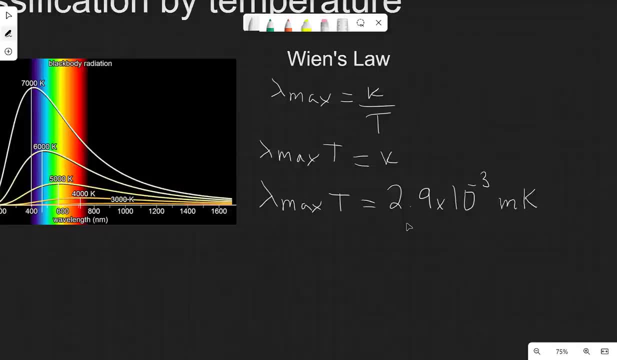 measured in meters Kelvin is equal to the temperature, and this has to be measured in kelvin, otherwise it will not work, so it will be meters kelvin will be meters kelvin. now it's really, really important not to confuse this with millikelvin, so I'm 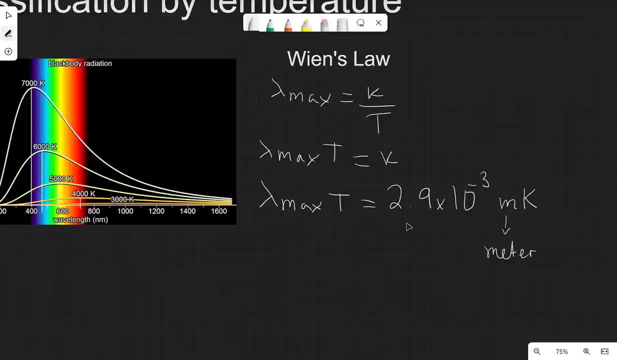 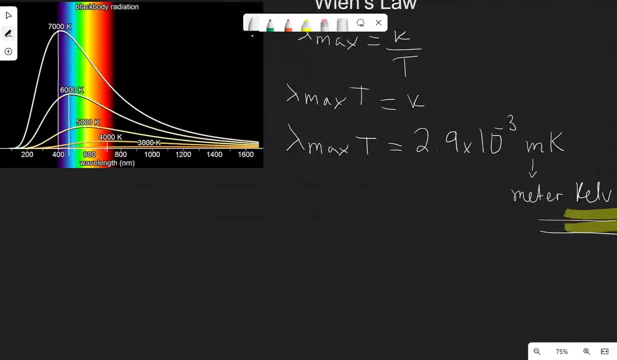 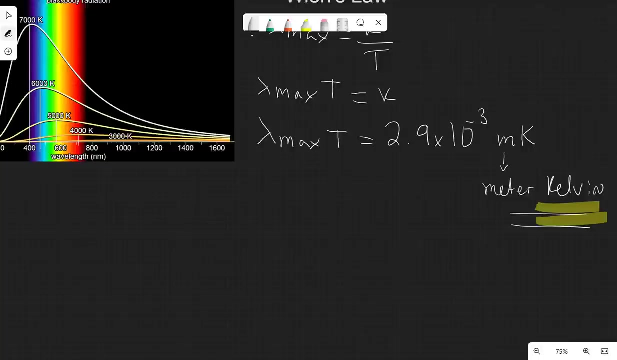 going to write it out in words underneath it's meter: Kelvin. your equation will not work in degrees Celsius, so I'm going to underline the Kelvin here. I'm going to show you a really, really important trick as well: if we're comparing two objects and we have just one unknown, we can also always say: 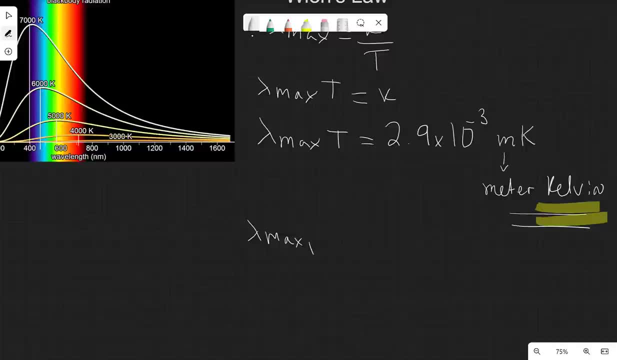 that lambda max 1 multiplied by t1 will be equal to lambda max 2 multiplied by t2. let's say we're trying. let's say that we have the predominant wavelength of one star and its temperature and we have the wavelength of the other star, but we need 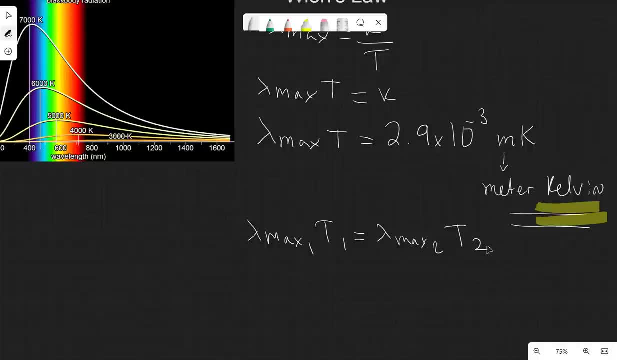 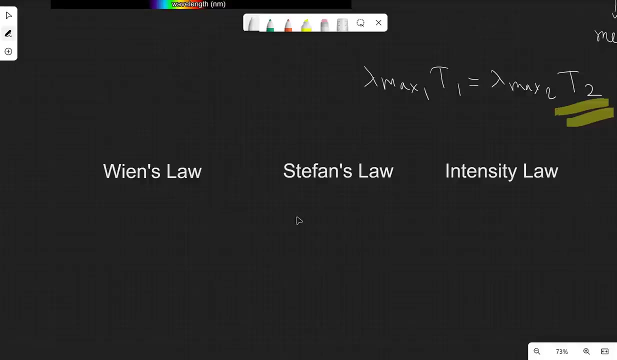 to find the temperature of the other star, then all we need to do is just directly rearrange this equation for t2 or any other unknown that is required. so in this portion of the spec we tend to combine, we tend to get a combination of those three laws. we have Venus law, which 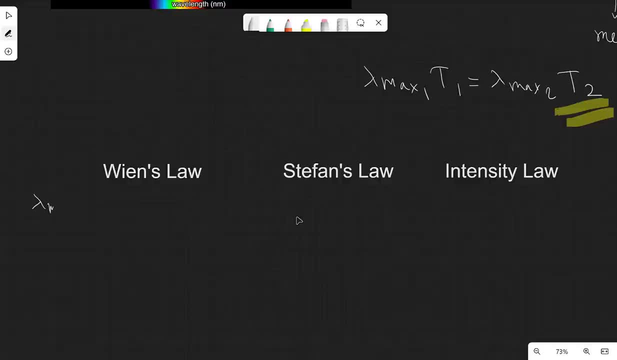 we've just introduced. let's just write that one more time for completeness. so the peak wavelength multiplied by the temperature is going to give us a constant 2.9 times 10 to the power of minus 3 meter Kelvin. we have Stefan's law, but that is all about the total outward radiated power by the star, sometimes in 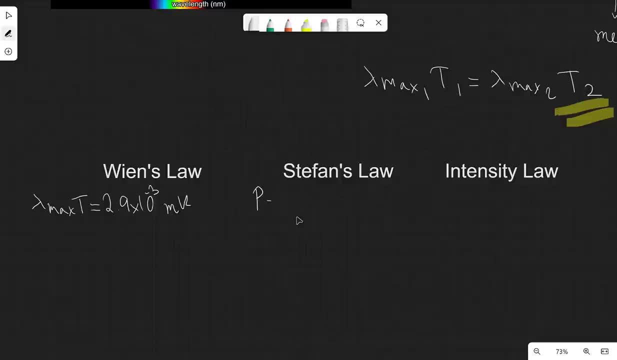 the books you may come across this written with the symbol for lunacity, L. but the total power which is gonna give it P now is equal to Stefan Boltzmann's constant, which has a value multiplied by the surface area of the star, multiplied by the temperature, raised to a power of four. now, typically in this equation, 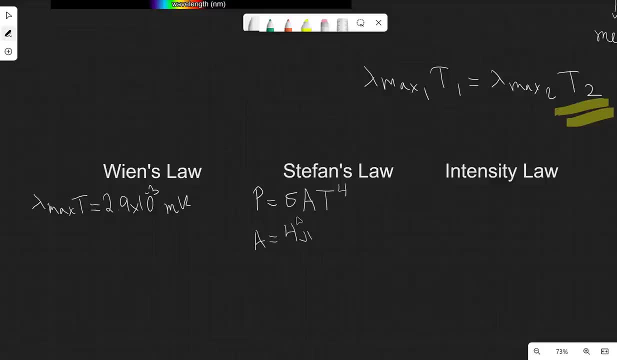 equation in the a is the surface area of a star or a different object, which is going to be given by 4 pi r squared. stefan boltzmann's constant just has a value: it's 5.67 times 10 to the power of. 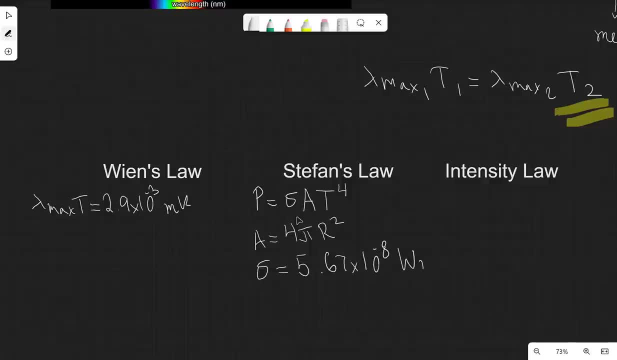 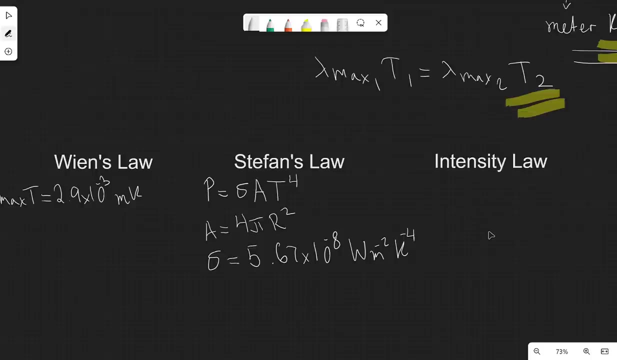 minus 8, and its units are going to be watts. m to the minus 2 k, to the power of minus 4. you also have the intensity law, which will give us the intensity at a distance away from the source, which is typically taught when we study waves. but intensity is equal to the power divided by: 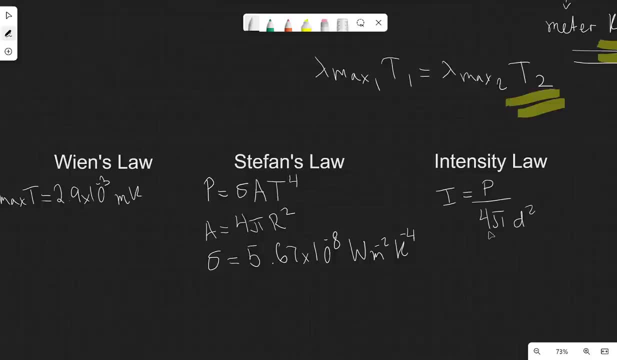 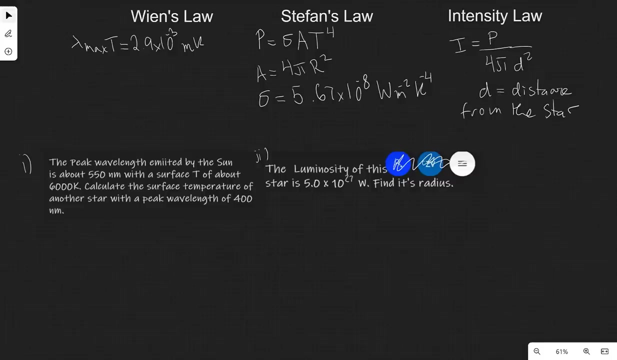 4 pi d squared, where d, in this case, will be the distance from the star to the observer. so let's just call it the distance from the star, whatever other object it is that we're dealing with, and typically we have to make a combination of those three equations, and let's apply this to an example problem. so first of all, 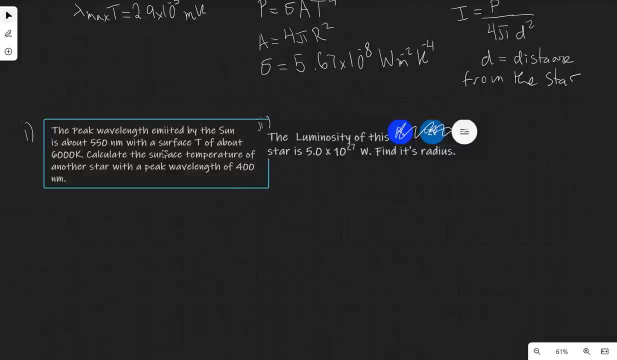 we have. the peak wavelength emitted by the sun is around 550 nanometers, but a surface temperature of around 6000 kelvin. calculate the surface temperature of another star with a peak wavelength of 400 nanometers. okay, so i'm going to use the good old technique that lambda max times t is. 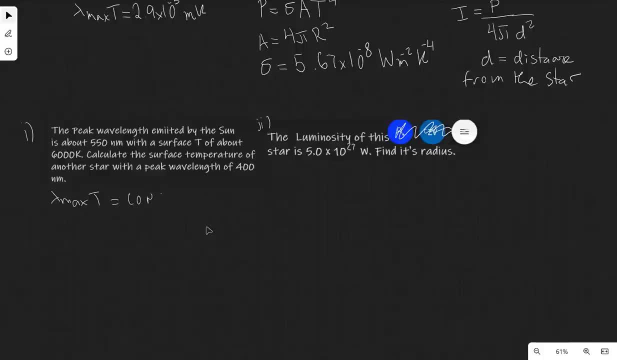 equal to a constant and don't even need to use the constant value. so i'm going to say that i'm going to say that lambda 1 t1 is equal to lambda 2 t2. so a typical trick, by the way, i've not included. 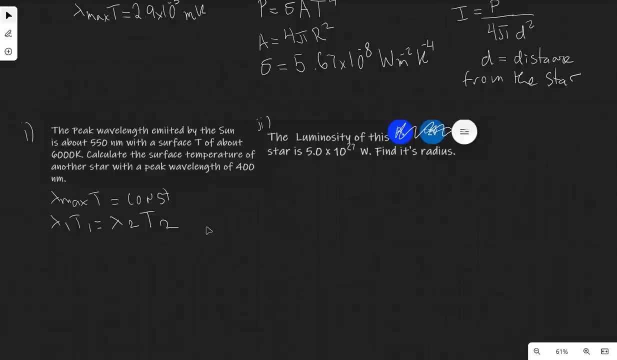 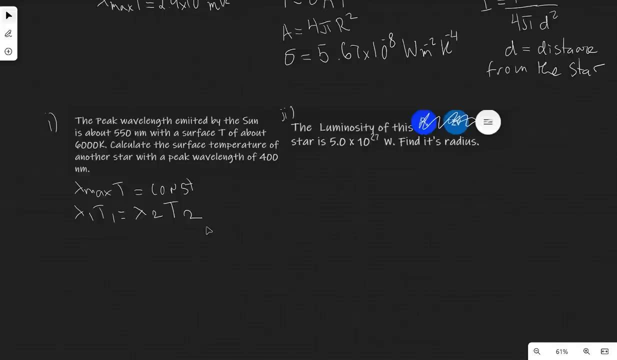 in this question would be to give you the temperature in celsius- make sure that it's in kelvin, please- and we can directly rearrange for the surface temperature of the second star, which is t2, which will be equal to lambda 1. t1 divided by lambda 2, so t2 will be equal to 550 nanometers. 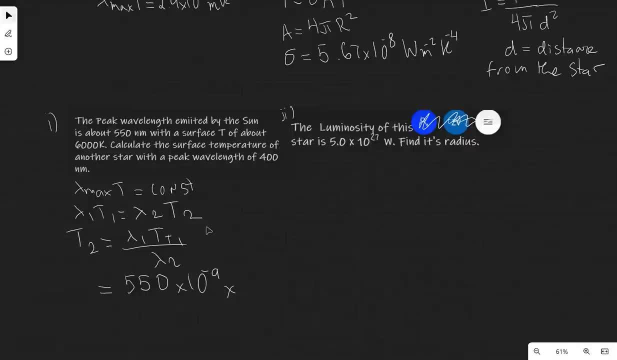 times 10 to the power of minus 9, multiplied by the surface temperature of the sun, which is around 6000 kelvin. then we're going to divide that by 400, which is our lambda 2 times 10 to the power hour minus 9. notice that because it's a ratio, the nanoprefix cancels we. 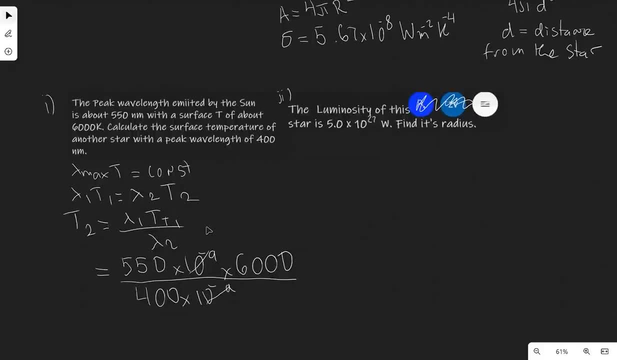 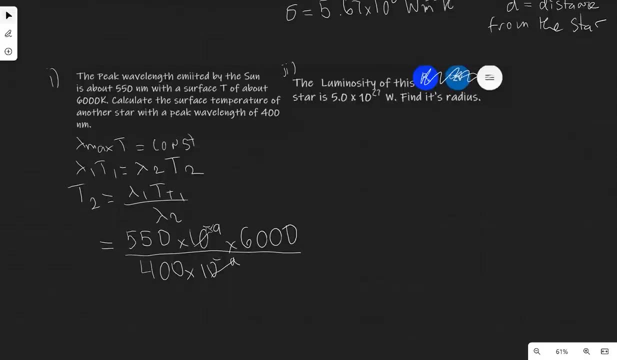 when it comes to an off article, i do like to write it here: t, so it's kind of like rub-k. so if you come back in the application, it's arms bar. so what's the Federal Plan? it has this basic: all номinals okay, and if we put that into a calculater we're going to get around a thousand. 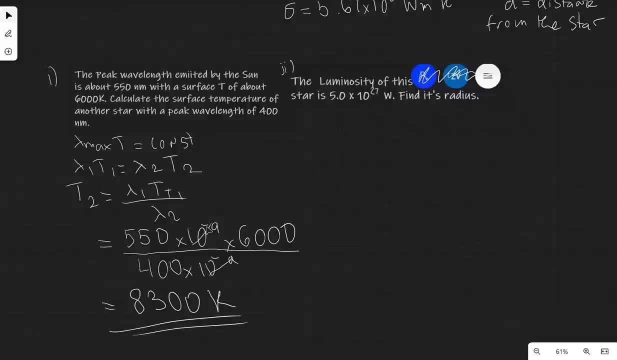 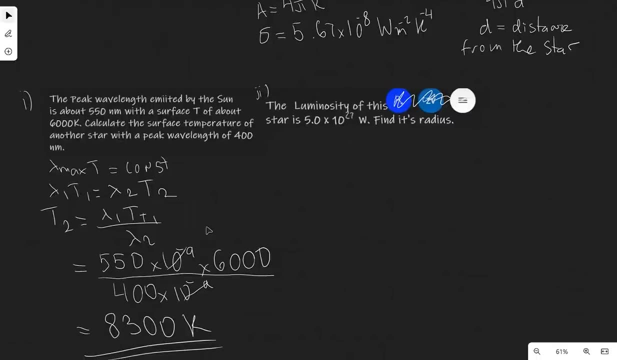 because it's a ratio the nanoprecance holds. we shouldn't even write it just to save time in this. for the temperature: Okay, now that we have that number for part 2, we can actually calculate its radius, because we're given its luminosity. 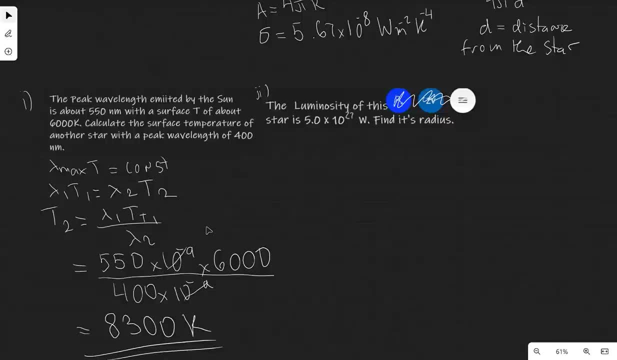 Now, remember the luminosity is the total power of the star and we can use the power equation, which is Stefan's law, which is going to be the constant multiplied by the area of the star, multiplied by T, to the power of 4, to calculate its radius. Well, remember the surface. 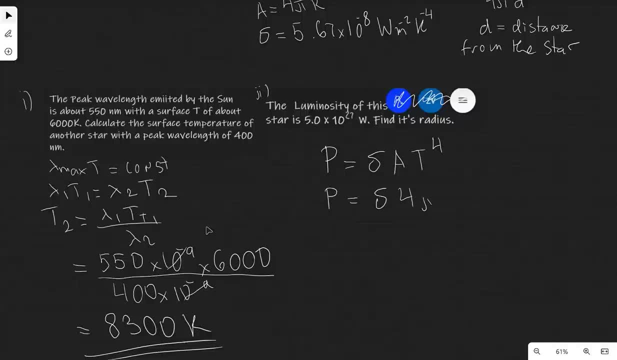 area is just equal to 4 pi r squared. so in this case we're just going to be looking for the radius and we can just directly rearrange for that. The radius will be given by the square root of the power and then we're going to be dividing that. 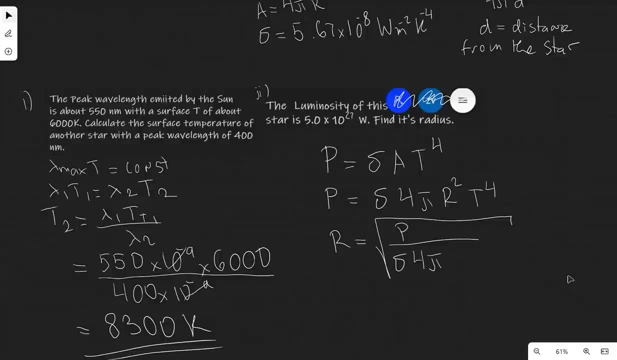 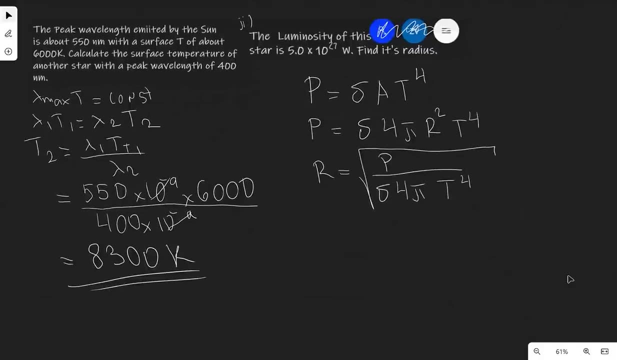 by the constant, and then 4 pi, and then what have we got left? T to the power of 4.. Well, let's plug in some numbers here. This is going to be kind of a long expression. The luminosity of the star is 5.0. 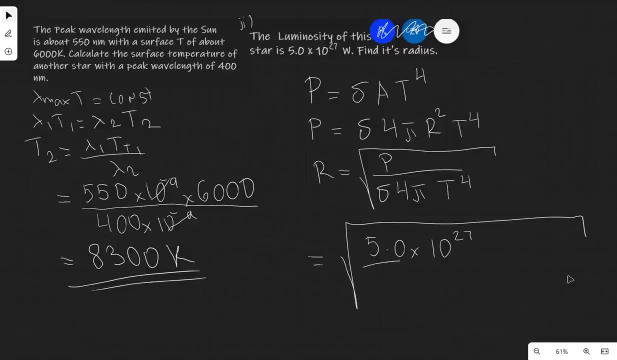 x 10 to the power of 27. then we're going to be dividing that by Stefan Boltzmann's constant, 5.67 times 10 to the power of minus 8.. 8- that's this guy here, multiplied by 4 pi, and then the temperature of the second star that we've. 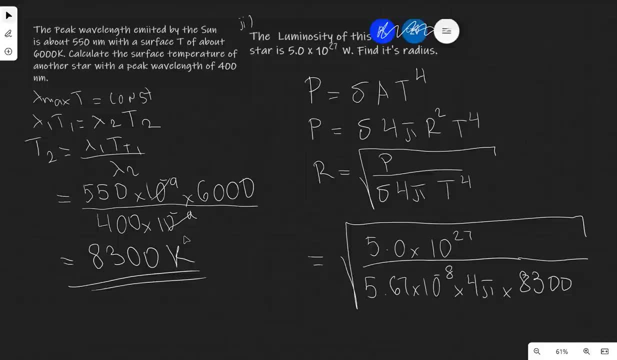 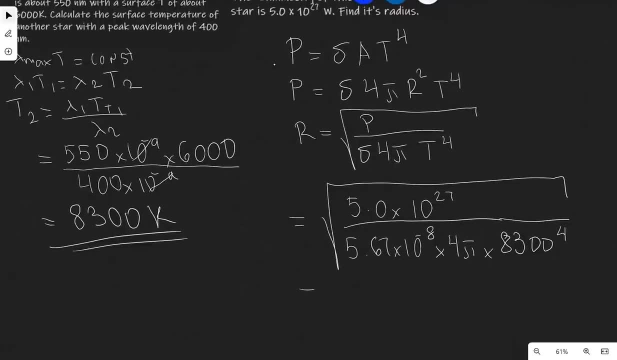 just found was 8300. very typical mistake for getting to raise that to the power of 4. and if we plug this into a calculator we're going to get around 1.2 times 10 to the 9 meters for the radius of the star. let's talk about spectra for a moment. the electrons can. 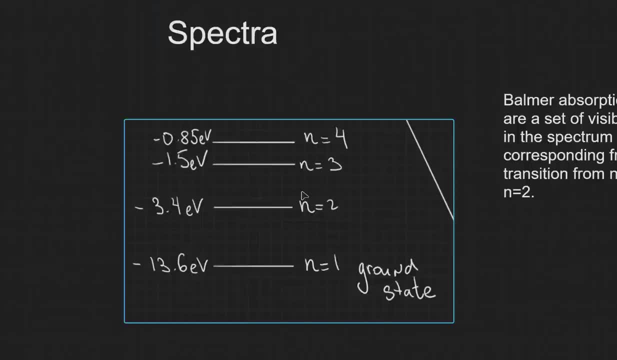 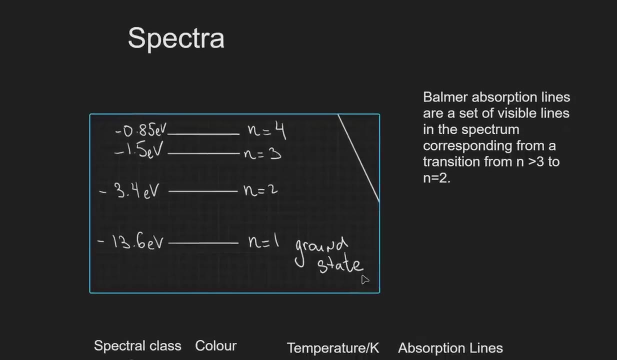 only exist in a set of defined energies around the nucleus. i have a really detailed video about this, including absorption emission spectra, which i'm going to link in the description which i go over this in a lot more detail now. the most negative state is known as the ground state. 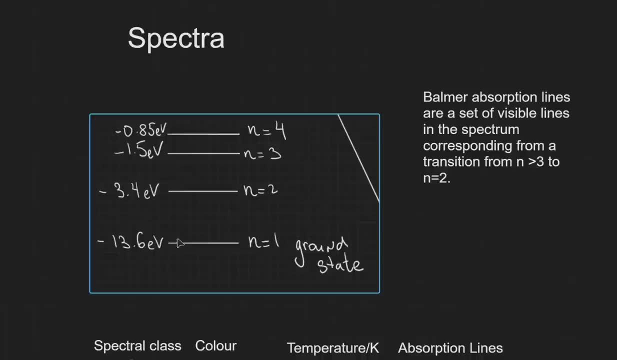 that is typically given. n is equal to 1. sometimes in a question, if we have to do a calculation, they will be given in electron volts. just make sure to convert those to joules. now there's a set of visible lines that are emitted, or a set of missing lines, when photons are absorbed, and the reason for that is because if an 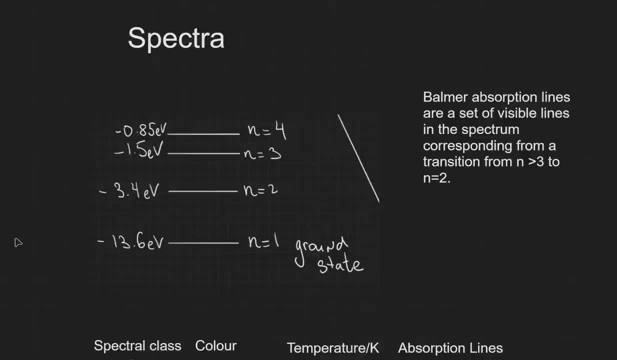 electron goes down in energy level. so let's say that we have a particle at n is equal to 4, then it goes down to n is equal to 2, then a photon will be emitted and the energy of that photon will be given by hf, where f is the frequency. it will basically correspond to some color, okay. 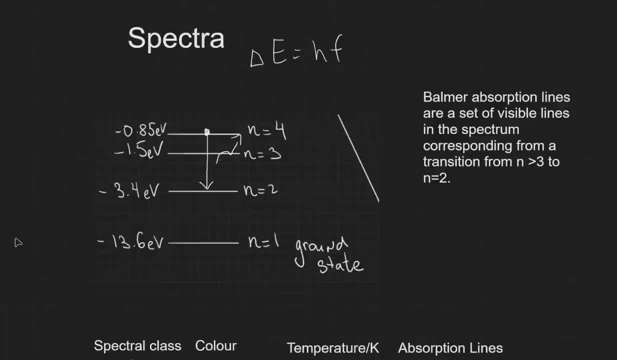 the opposite will happen if a photon is absorbed, and that's how an emission and an absorption spectra is formed. now there's a set of lines which are known as the ground state, and they're known as the baumer absorption lines, and they correspond from a transition from n is equal or. 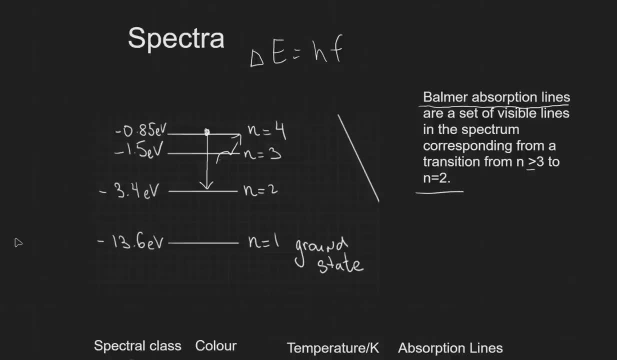 greater than 3 to n is equal to 2.. in other words, um, it will be a spectrum, a set of lines that are gonna, that are going to correspond from, and it's equal to four, two and six equal to two. from n is equal to three. then from the higher energy levels as well, which I've not drawn here back down to, and is equal 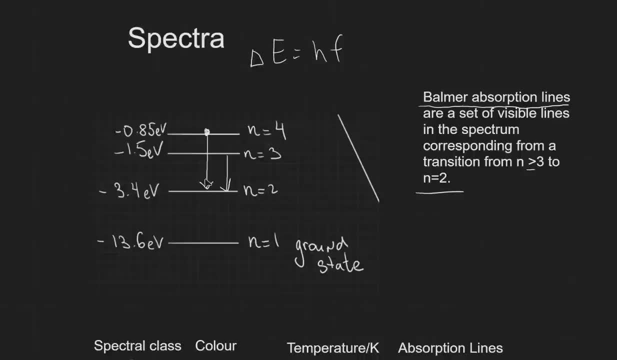 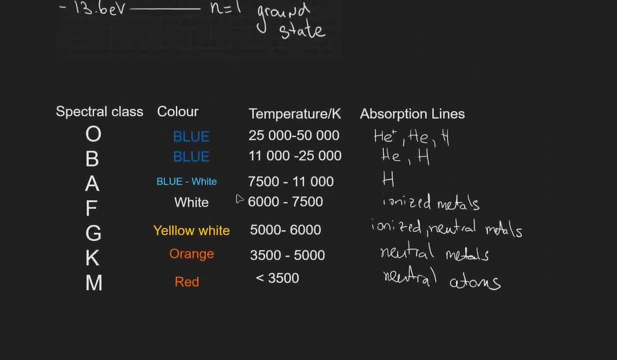 to 2 than from the higher energy levels as well, which I have not drawn here- concepts, as shown here in the diagram, equal to 2.. Okay, now, the next thing that we're going to be talking about are the spectral classes of stars and this table. we need to remember the characteristics. 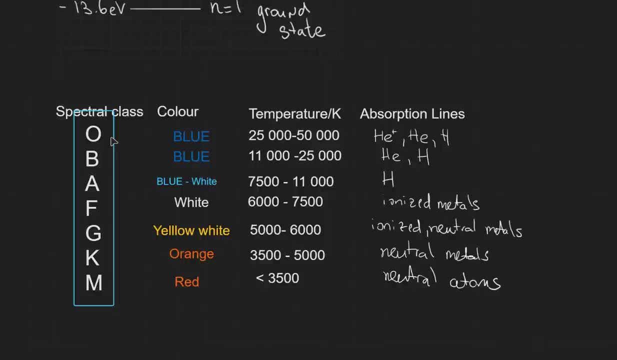 for. So the spectral classes are given names O, B, A, F, G, K and M, and you can use your favorite method of remembering this. They're going to correspond to a different color. They will be going with the spectrum. so we're going to start off. 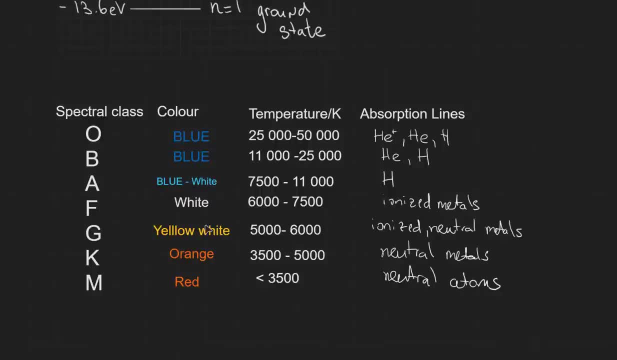 with blue and then we're going to move into blue, white, then white and then yellow, white and then orange and then finally red. Remember, red has the longest wavelength and hence the lowest temperature. It's kind of useful to remember that our Sun is sort of yellow white, and that corresponds to around 5. 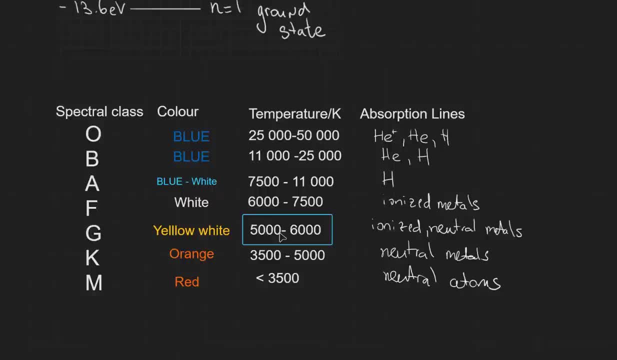 between 5 and 6,000 Kelvin. Well, the surface temperature is close to 6,000. that's a different story. So we're going to start off with blue and then we're going to move into blue, white and then yellow, white and then orange and then finally red. Remember, red has the longest wavelength and hence the lowest temperature. It's kind of useful to remember that our Sun is sort of yellow white and that corresponds to around 5, between 5 and 6,000 Kelvin. Well, the surface temperature is close to 6,000. that's a different story. 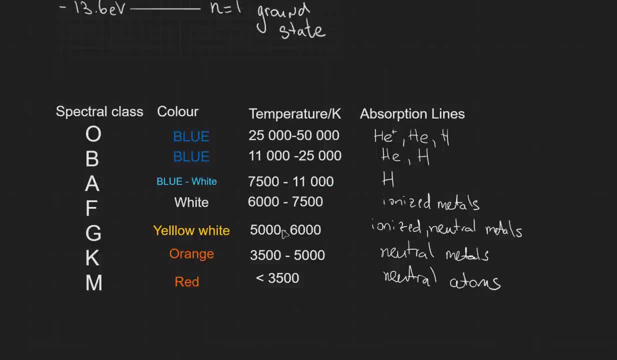 But we're going to need to find a way of remembering these values. In terms of the absorption lines of the Balmer spectrum, different things will be absorbed, which will tell us what's essentially what the main composition of the star is that I've listed over here. So we have things like helium hydrogen. 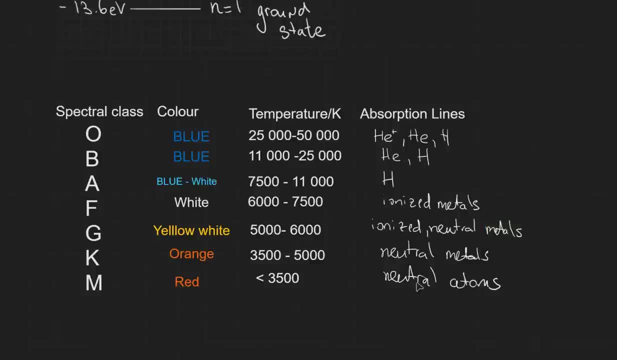 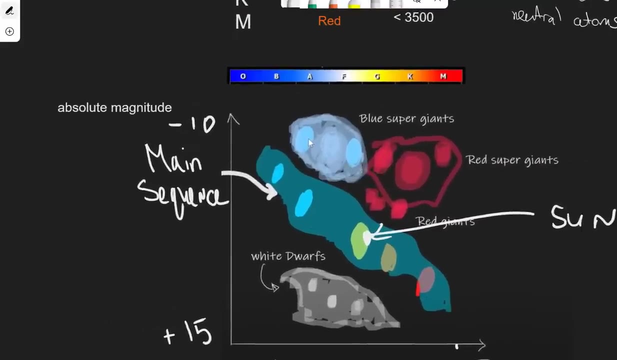 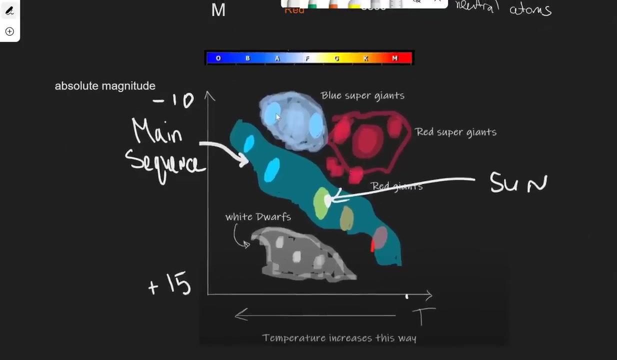 ionized metals, ionized metals, neutral metals and in the stars which have the lowest temperature, it will be neutral atoms. Another way of classifying the stars is using this diagram here, which is known as an HR diagram or a Hertzsprung-Russell diagram. So what are? 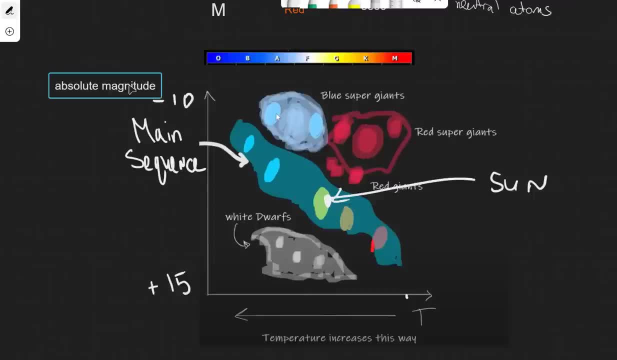 the main points. First of all, on the y-axis, we have absolute magnitude, and this tends to range from around minus 10 at the highest. Remember, a high negative absolute magnitude means a very bright object, So something like a blue giant, for instance, Whereas on the other hand, we're 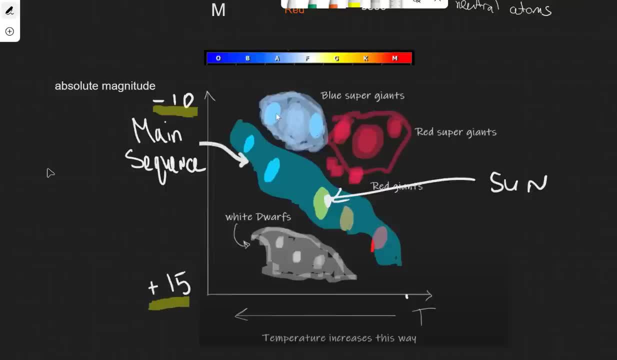 going to have some very faint objects with an absolute magnitude of around plus 15.. Another highlight is that the temperature increases the opposite way, and this is really, really important. We need to remember the ranges of the scale, so it'll go somewhere from around 50,000 or so Kelvin up to a 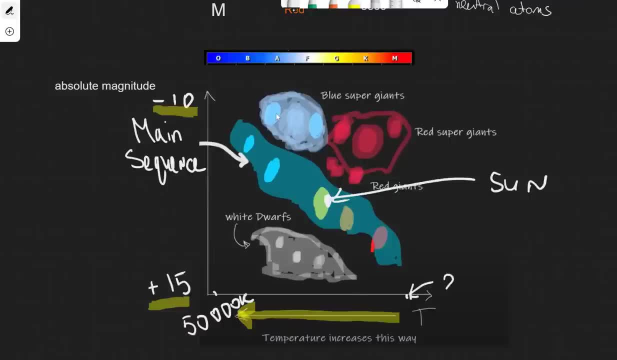 little bit higher than that. So let's take a look at the position of the sun. So the position of the sun is right around here. Notice that right at the top we also have the spectral classifications of stars, as we discussed in the table up here. So 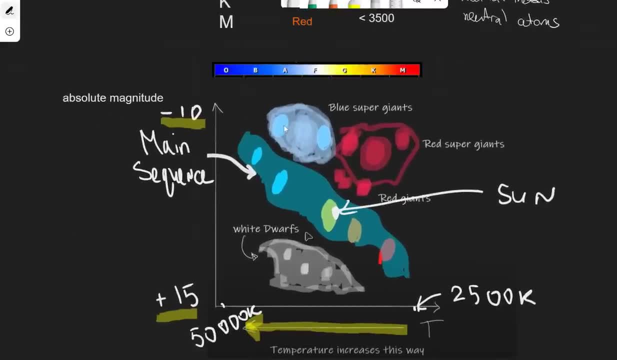 O, B, A, F, G, K and M. Then here is the position of the sun. Okay, well, what will happen to our sun as it's evolving? Remember, when the sun loses its hydrogen fuel, it will eventually turn into a red giant. The red giant's region is right across. 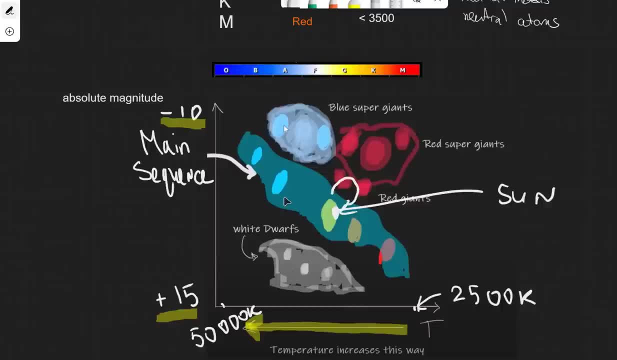 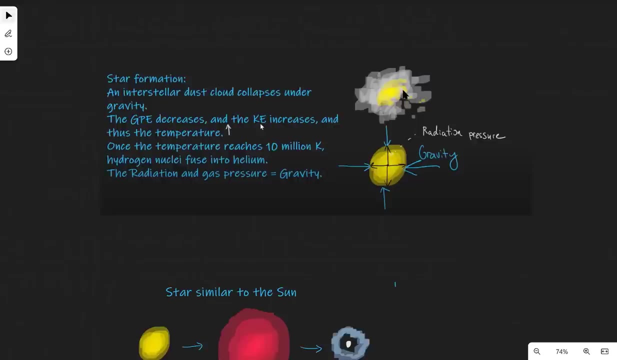 here and after it becomes a red giant, it will end up being a white dwarf eventually, So it will move to this part of the diagram. So how is the star actually formed? Well, we have an interstellar dust cloud that tends to collapse under gravity, the gravitational potential. 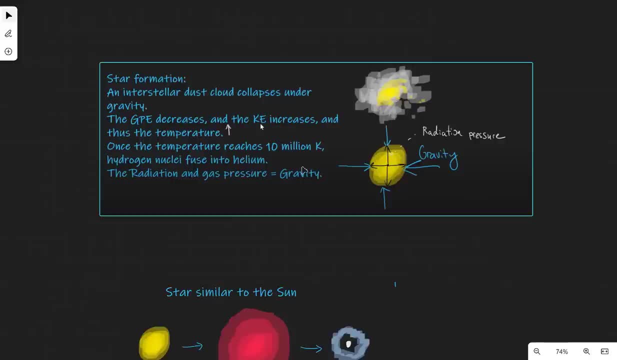 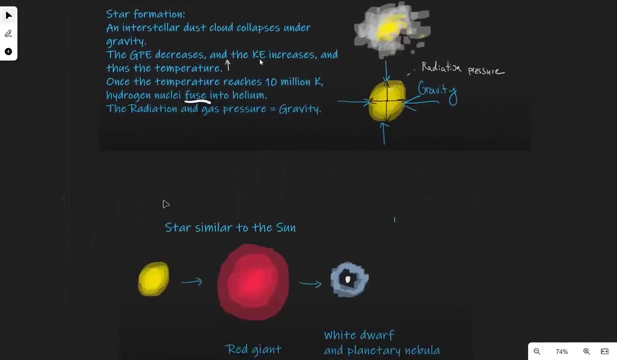 energy decreases. the temperature increases around 10 million Kelvin, We don't really need to remember the number. The nuclei, the hydrogen nuclei, starts to start to fuse into helium, and the word fuse here is critical. This is what actually gives the energy of the star. What is the evolution of a star that is? 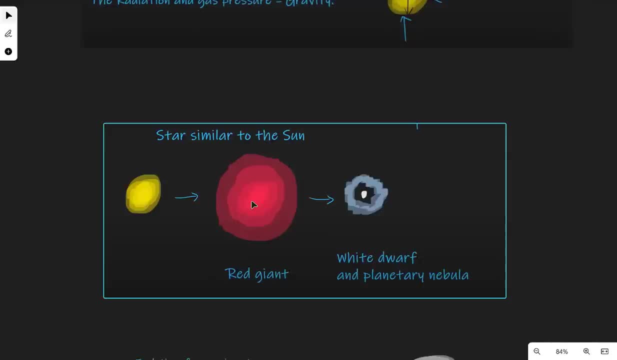 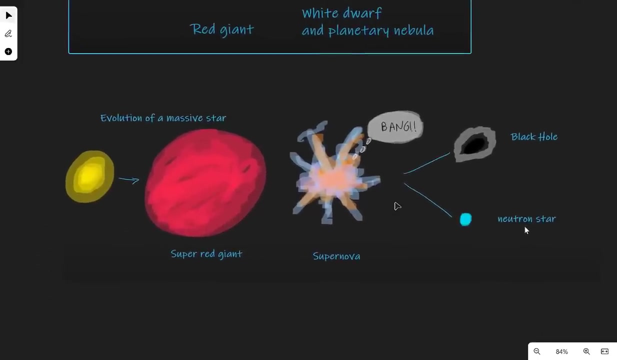 similar to the Sun. Well, our Sun will turn into a red giant, as we've just shown on the HR diagram, and then it will eventually turn into a white dwarf with a planetary nebula. A much more massive star will undergo a very different life cycle, So it will turn into a super red giant. so a 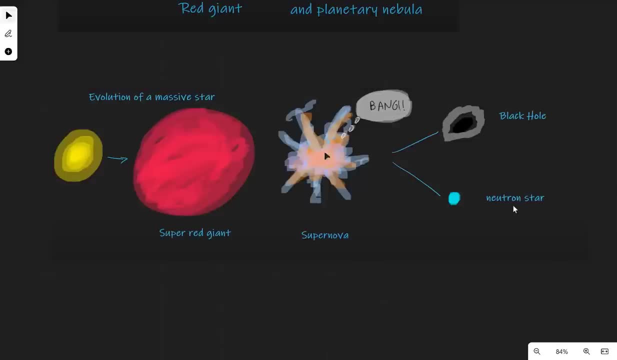 little bit further left on the HR diagram, but then it will cause one of the biggest explosions in the universe, which is a supernova. This is not up to scale. These things have a lot of energy and they're not going to be able to. 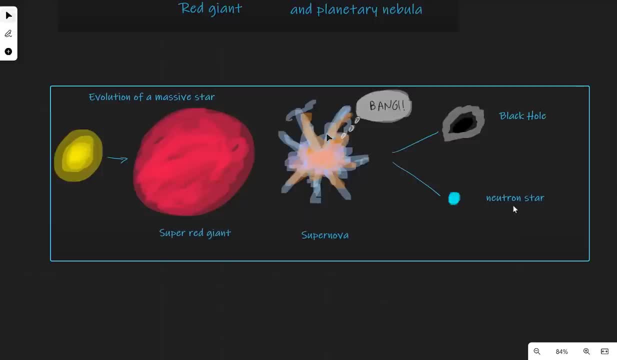 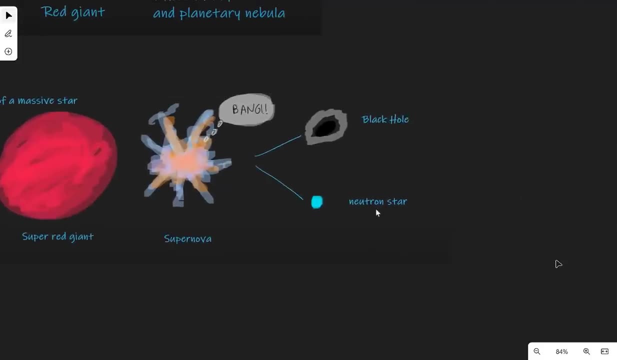 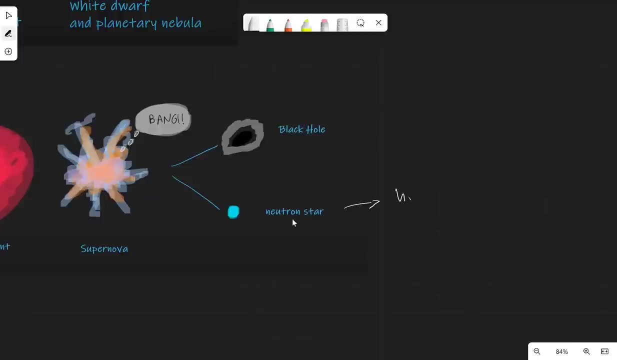 have a huge absolute magnitude that out shines an entire galaxy. Depending on the mass of the star, then it will turn either into a neutron star or a black hole. What are the characteristics of a neutron star? Well, it will have an incredibly high density. We're talking of the order of four, sometimes higher times. 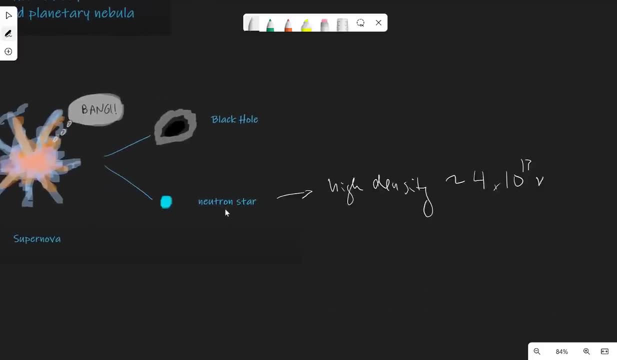 ten to the power of seventeen kilograms per cubic meter, Which is very, very similar to the density of the nucleus itself. So we have, essentially, neutrons that are as tightly packed as they possibly could be. They have a very small size. They're of the order of literally around ten miles. so 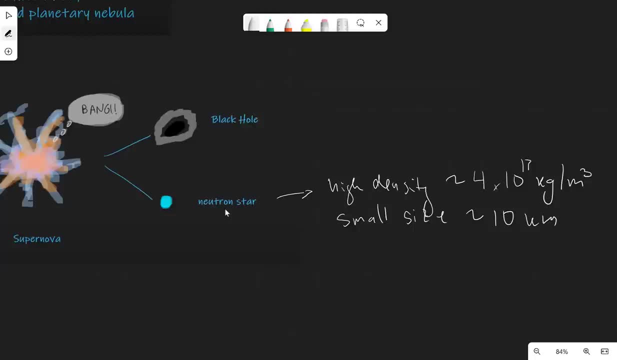 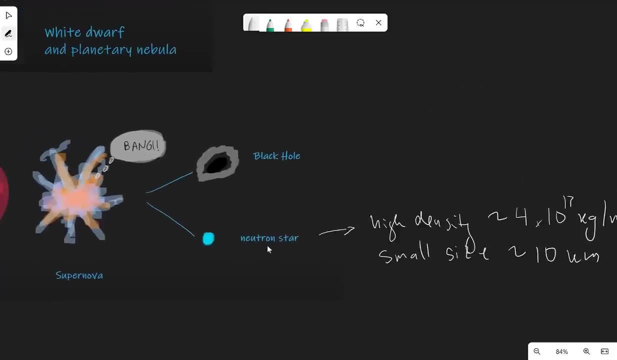 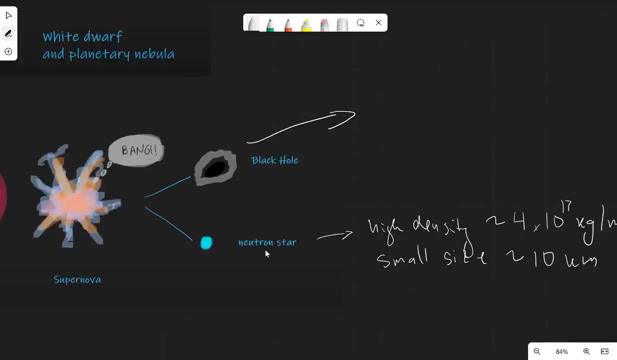 should we just say around ten kilometers or so, Something of the mass of the Sun that's been squashed to the, to the size of a small city In terms of a black hole, the really really interesting object in the universe. they're so incredibly dense that the escape velocity is higher than 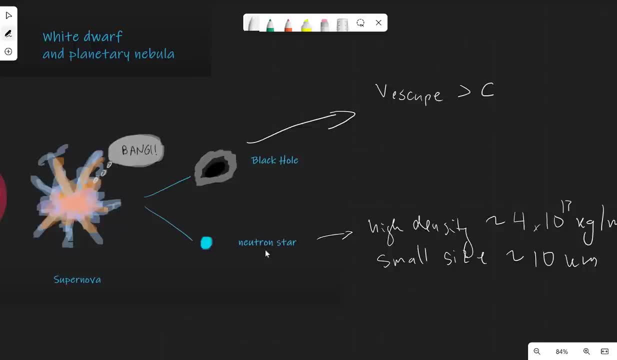 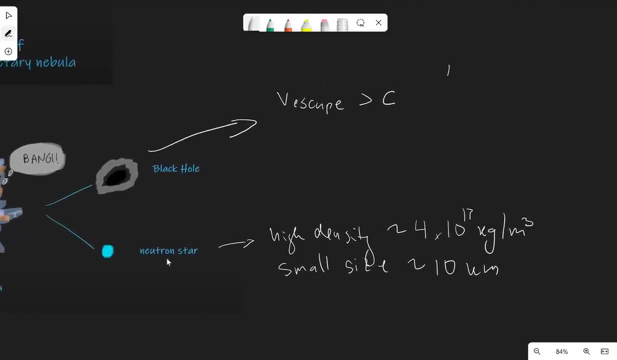 the speed of light. We can also find the Schwarzschild radius for the formation of a black hole. The way we do that is by setting the kinetic energy equal to the gravitational potential energy. So that's how we find the escape velocity. We should just call that VE, where M is the mass of the object, that's. 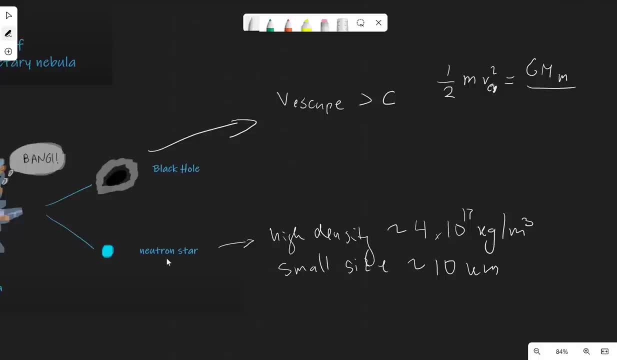 being turned into a black hole. And then we're going to be dividing this by the radius and I'm going to call this radius RS, where S stands for the Schwarzschild radius. So M is going to cancel out, and then I'm going to say that the 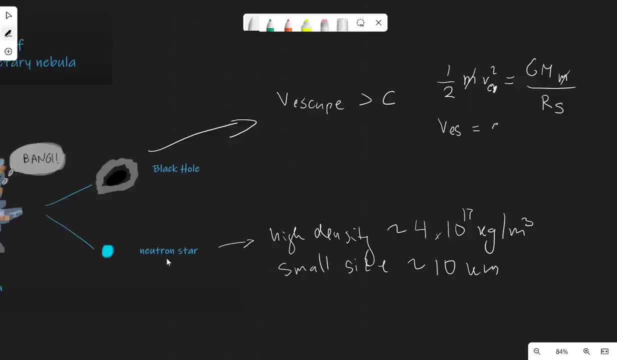 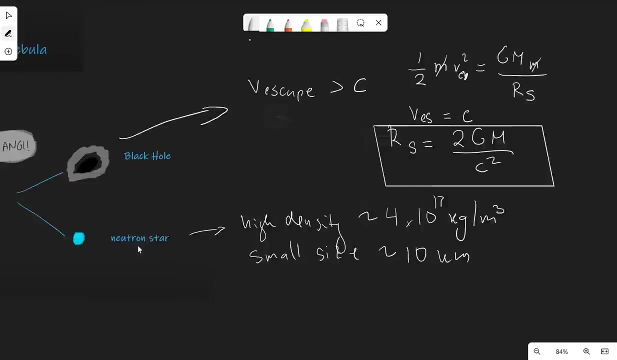 the escape velocity is actually equal to c and just rearranging for the schwarzschild radius we're going to get that this will be equal to 2 g m divided by the escape velocity squared. but this is now just c and this will be c squared. so this here is the formula for the schwarz. 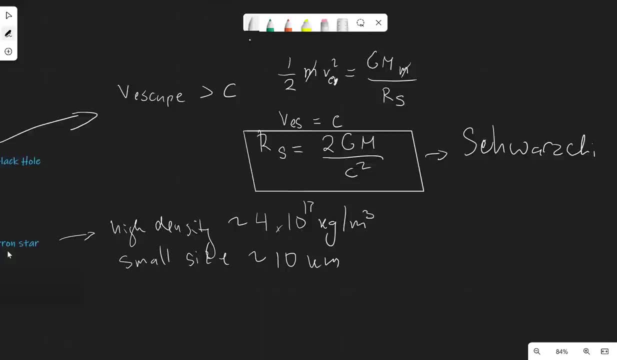 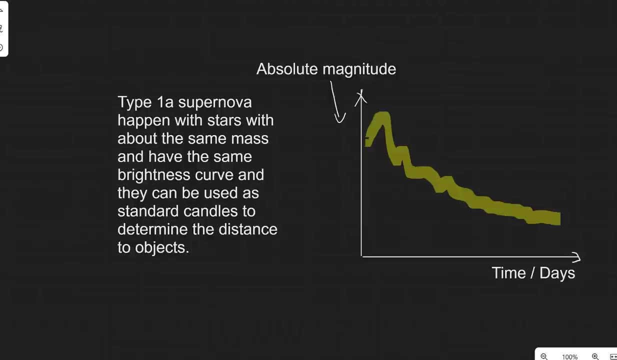 see if i can spell it correctly: child radius. if we compare something to the size of this, it is going to form a black hole. we also need to mention type 1 supernovae, which happen with stars which have roughly the same mass and the same brightness curve. they can be used as standard. 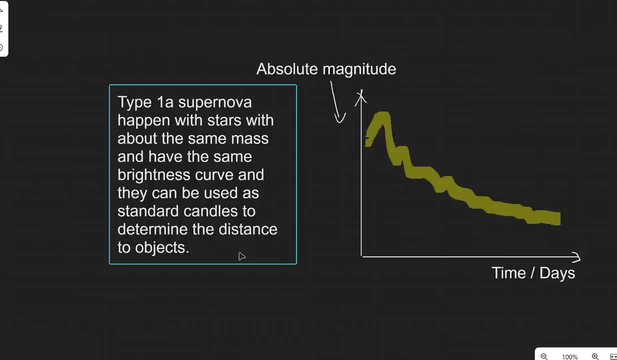 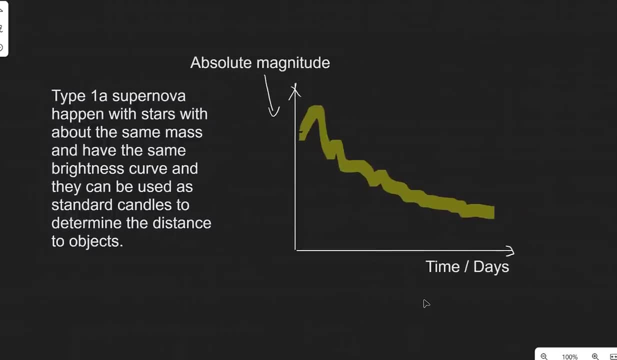 candles to determine the distance to objects. this actually became critical for our study of the universe. their absolute magnitude compared to time looks something like this: it's very, very high initially, tends to vary a little bit but in the way it's drawn. but very high initially and then gradually. 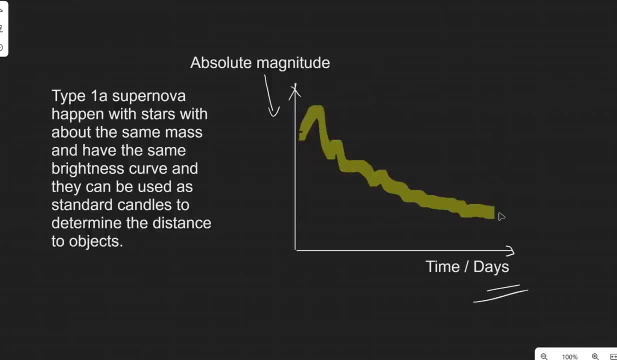 drops down over days. you may be asked to add in a unit, for instance in an exam, or they may try and trick you with the unit and find a mistake, etc. so it's important to know that this happens over days. they're so bright actually that they can even 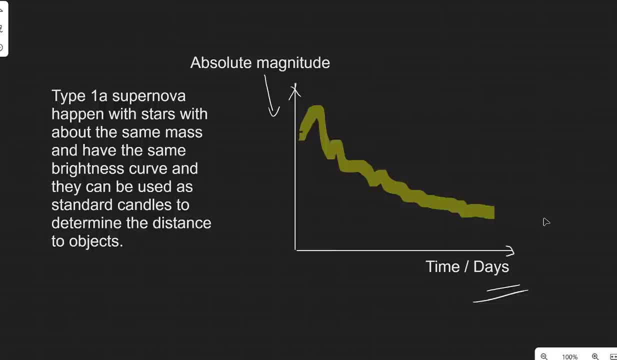 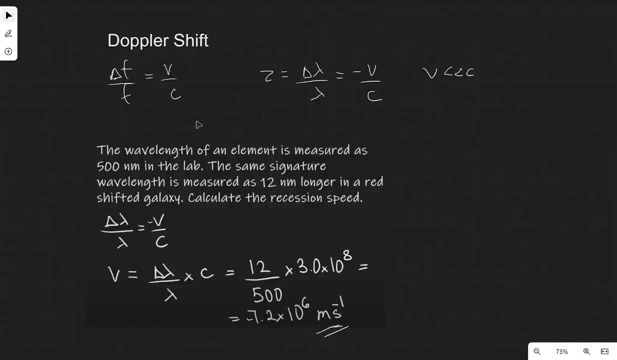 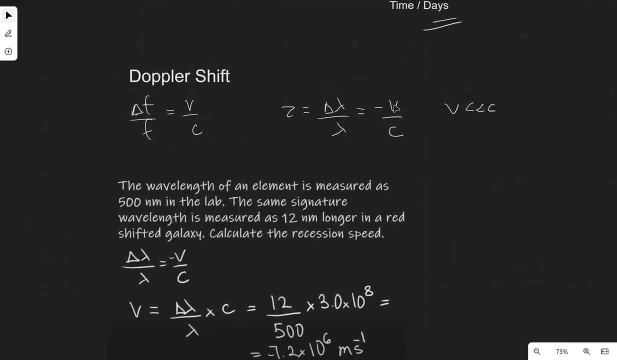 outshine almost an entire galaxy during this process. ok, were going to talk about the Doppler effect next, and that is the relative change in the frequency of the wavelength if the source is moving with respect to the observer south to us. dealt an F in this equation is change in frequency. 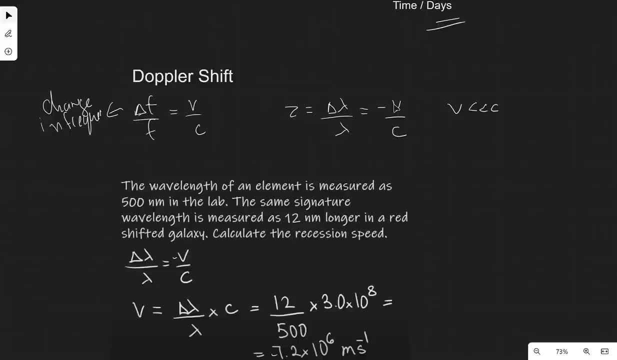 and and F. here is the frequency that changes from right to left in the frequency of a wave failure. реально does this change change? think you will actually know more about defined way in a moment because this later Ghonim is a Irakli obama and this uncertainty vehicle talks about, but 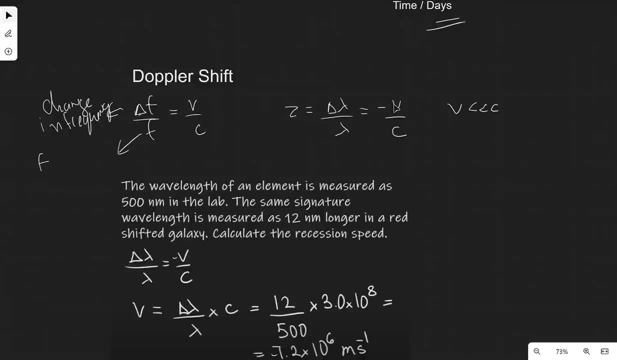 that was not conceptual distinguishing between function number one. he broke employment or frequency as measured in the lab. So this is really, really important. Okay, so this is equal to v, which is the relative speed between the source and the observer. We don't actually know. 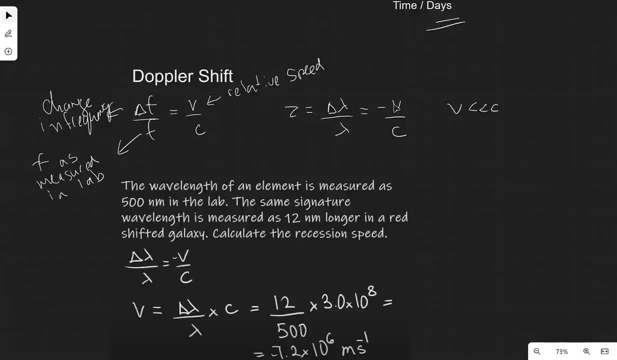 which one's moving, So I'm just going to call it the relative speed, And the c here is the speed of light. We can define a quantity which is known as the red shift, given the symbol z, And this is equal to, exactly same way, the fractional change in the wavelength. But we also get a minus sign. 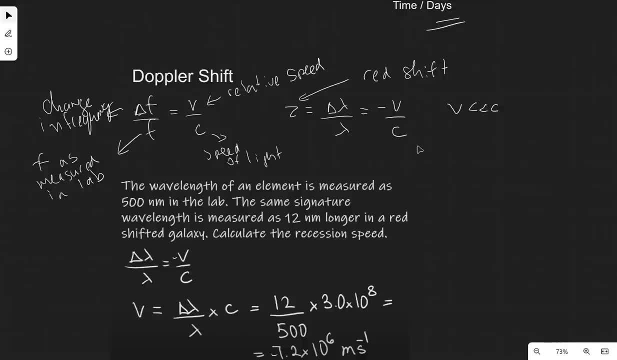 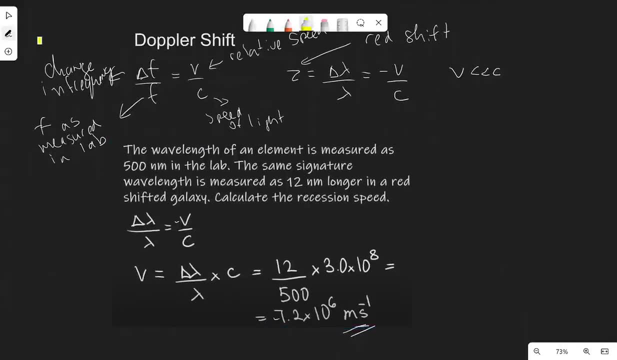 in front of here. Well, let me apply this to an example We have. the wavelength of an element is measured as 500 nanometers in the light, And this is the wavelength of an element. So this is the wavelength of an element, And this is the wavelength of an element. So this is the wavelength. 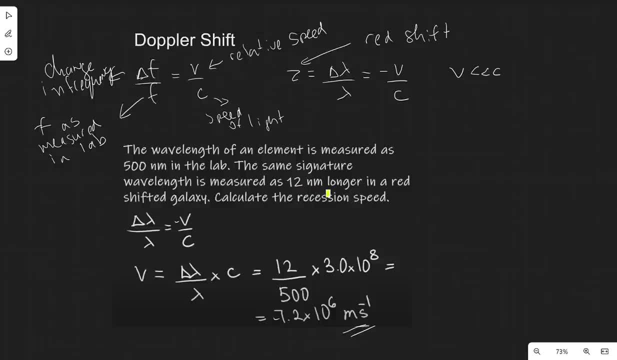 lab. the same signature wavelength is measures 12 nanometers longer in a red shifted galaxy. calculate the recession speed. okay, well, we just. all we need to do is just rearrange for v, and in this case this will be equal to the negative of delta lambda over lambda times delta c. okay so. 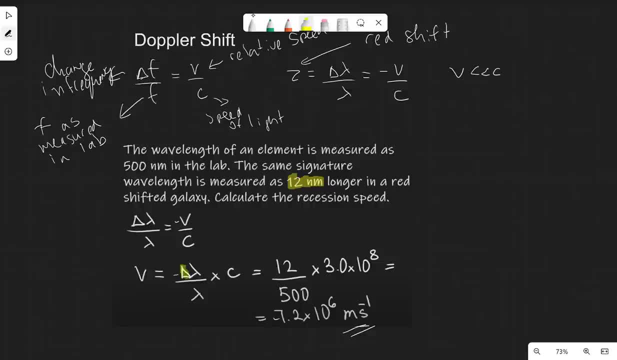 we know that our change in wavelength is going to be equal to 12. we know that our original wavelength was equal to 500 like. so we multiply that by the speed of light and we find a very high recession velocity for this galaxy, and this is a technique that will allow us to calculate the speed of 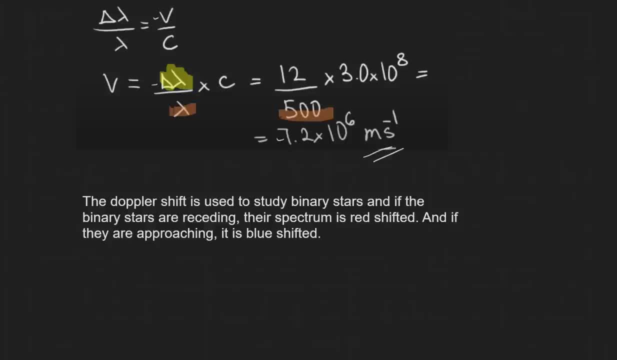 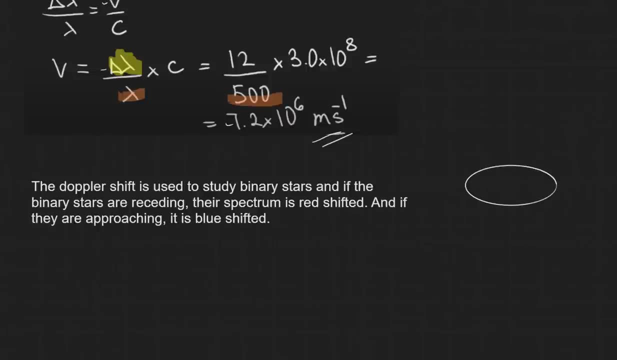 moving objects. the Doppler shift can also be applied to the study of binary stars, and most of the stars actually out there are binary. so let's say that we have a couple of stars that are orbiting one another, so at the moment when they are approaching us, if they're approaching us, then this means that 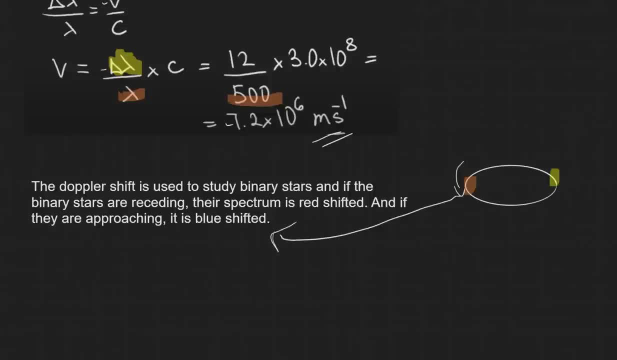 there will be blue shifted, whereas this one here, the red shifted. now, if we start the calculation, we'll see that the velocity of theлонwayc is different now, even on the position. if it is going this way, it will be moving away from us, and if 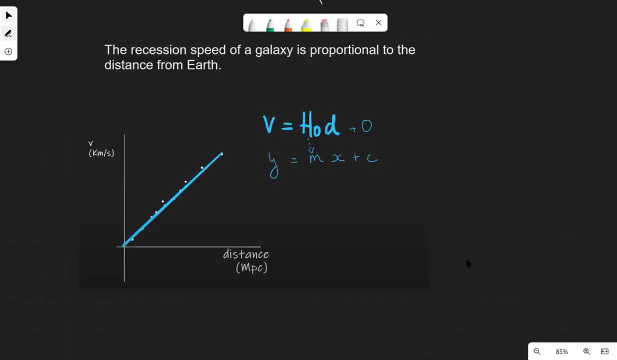 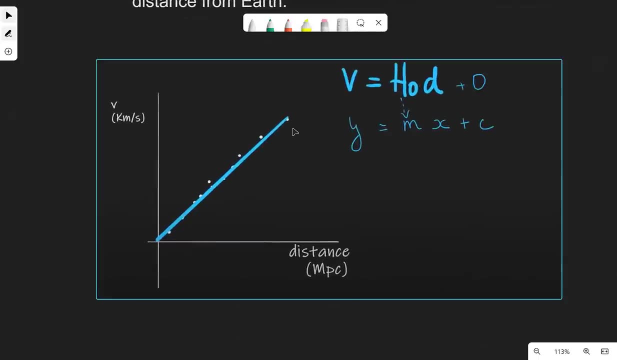 that's the case, it will be red shifted because it's receding. now, if we measure the recession velocity of all the galaxies out there, we find something absolutely remarkable. look at this straight line correlation. on the y-axis we have the velocity, the recession velocity, in collaboration with delta plus 1 and delta c, of the velocity of the galaxy in the galaxy equation. we can see that the velocity of the galaxy is very similar to the velocity of the galaxy equation in the galaxy equation and this is why this is very important. 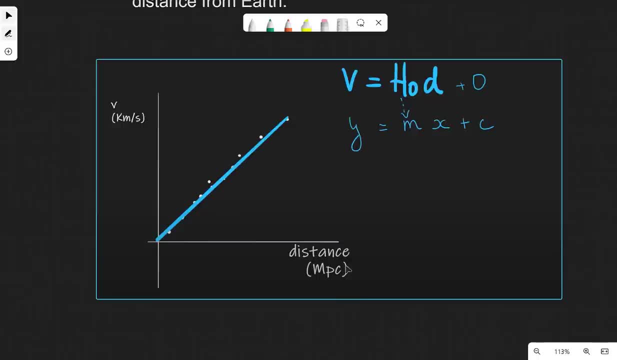 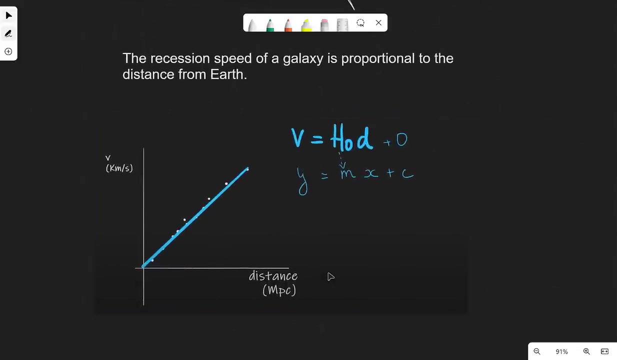 meters per second, and on the x-axis we have the distance in mega parsecs, we can see that the speed of the recession of the galaxy is proportional to its distance from earth, and this here is known as hubble's law. if we were to apply some y equals mx plus c analysis, and if v is on the y-axis, if 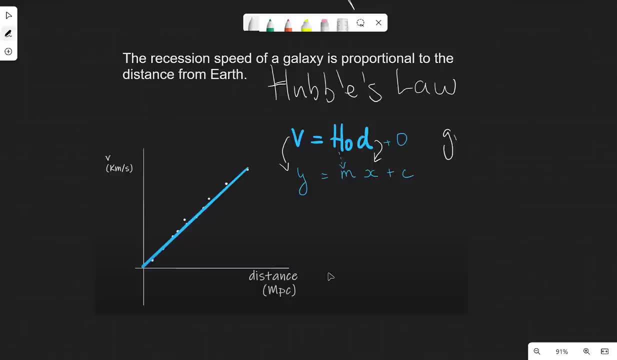 the distance is on the x-axis, then our gradient is equal to hubble's constant h naught. now if we do a little bit of maths, we're going to figure out that h naught will actually have units of speed over distance. well, speed is typically measured in meters per second. now we've got it in kilometers. 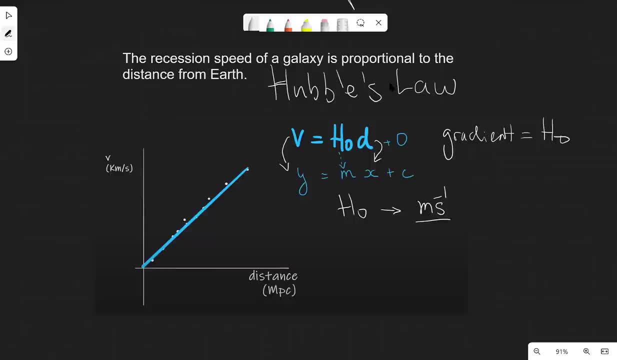 per second, but we're going to have to use the linear equation to explain the gradient of speed in real time. if we're going to do a little bit of math, we're going to have to use the linear equation. just speak in general. then we're going to be dividing that by distance. so the overall base 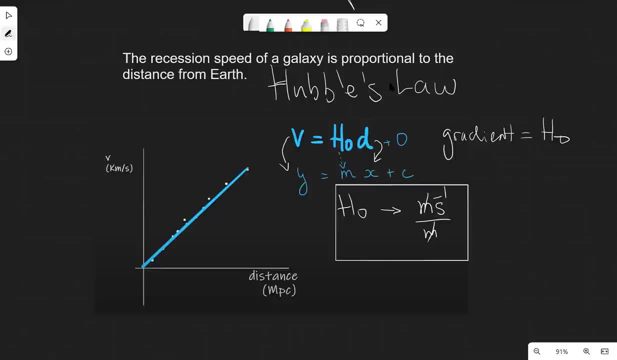 unit of h naught is one over seconds now. this means, though, that if we do one over h naught, then what we're going to get is something with units of seconds, with units of time, and this here means that we can essentially estimate the age of the universe, and this here is a very 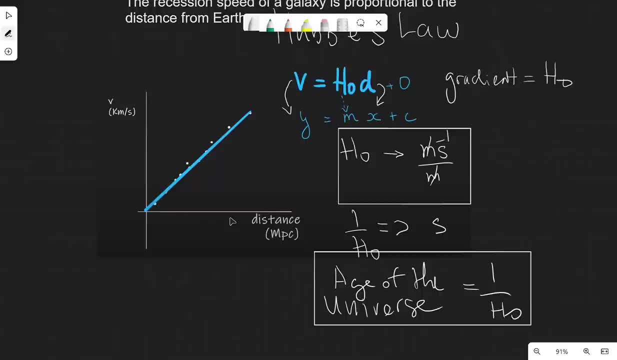 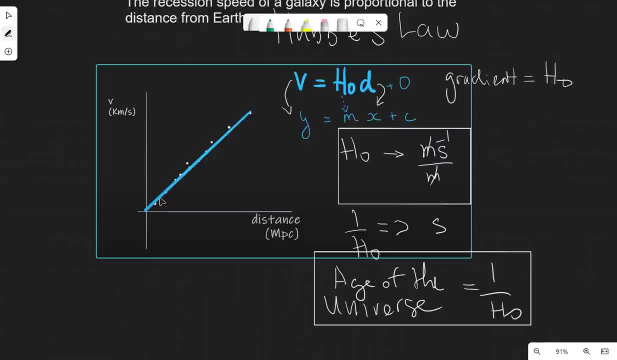 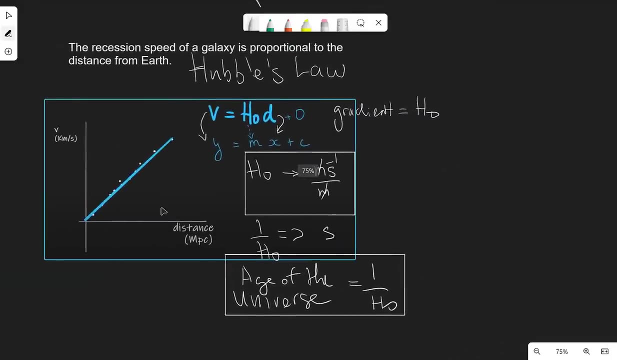 closer before and at some point we reach a time where all the galaxies were occupying the same region. i, i, i. this is the concept of the big bang. now, how can we actually calculate this time? well, observations show that the value of hubble's constant is somewhere around 70 kilometers per second. per. 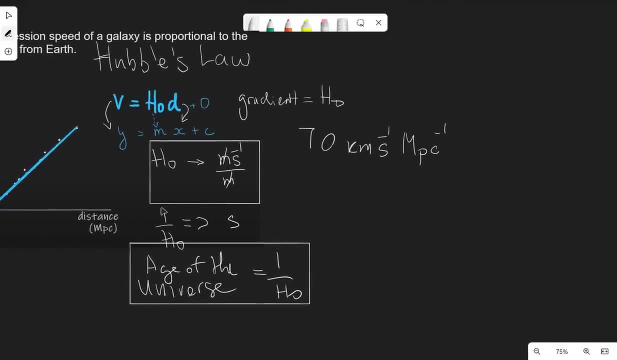 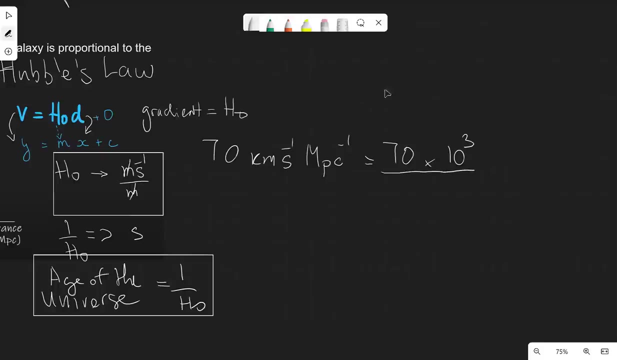 megaparsec. well, let's convert that to si units. the way we're going to do that is, first of all we're going to multiply by 10 to the 3, which is the kilometers part, and then we're dividing by an entire megaparsec. so this negative. 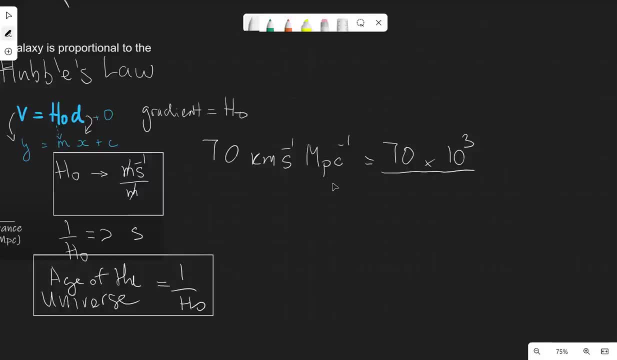 one applies to both the mega and the parsec. so we're going to divide by 10 to the 6, and also one parsec we're going to need to convert that to meters and that was around 3.08 multiplied by 10 to the power of 10, and that's going to be about 3.08, and that's going to be about 3.08. 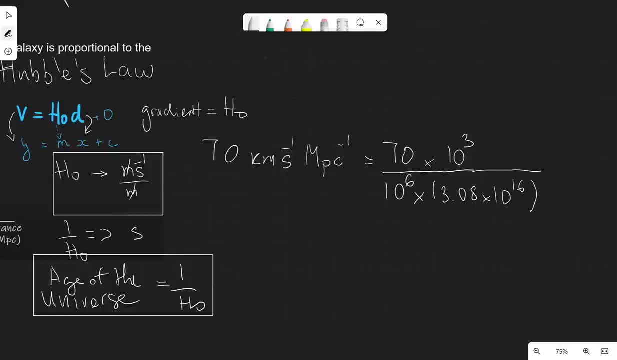 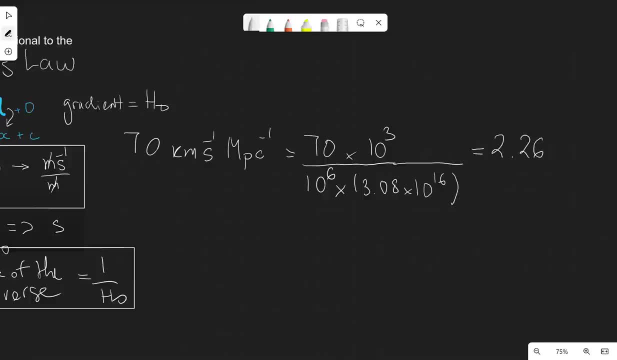 in si units to be around 2.26 multiplied by 10, raised to a power of minus 18, s to a power of minus 1.. now from this value we can actually calculate the age of the universe, which is just 1 over the value. so i'll be 1 over 2.26 times 10 to the power of minus 18. 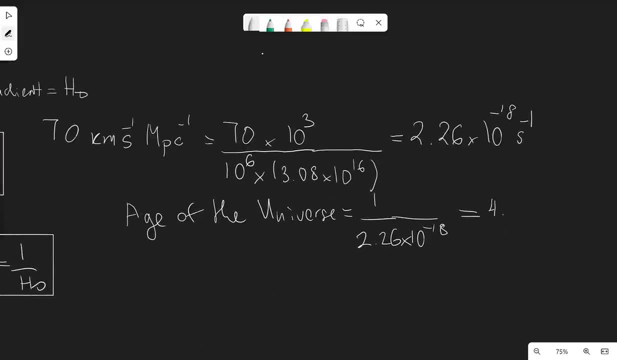 and if we were to put that into a calculator, we're going to get around 4.42 times 10, to the power of 17 seconds. now, that is a lot of seconds, but what is it in years? so, in order to find this, what i'm 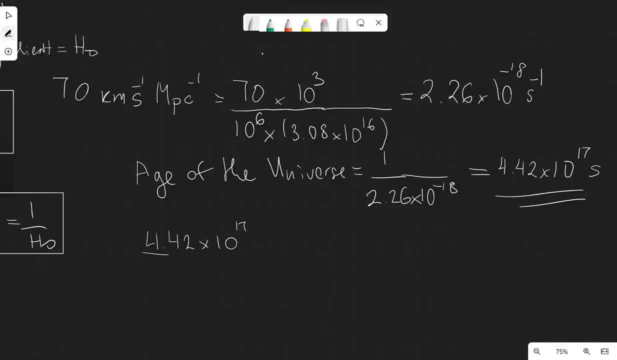 going to do is i'm going to divide that by the number of seconds that we're going to need to calculate the number of seconds in a year. so 3, 6, 5. each of them has 24 hours, each of them has 60 minutes times 60 seconds and if we put that into a calculator, we're going to get around 1.4 times. 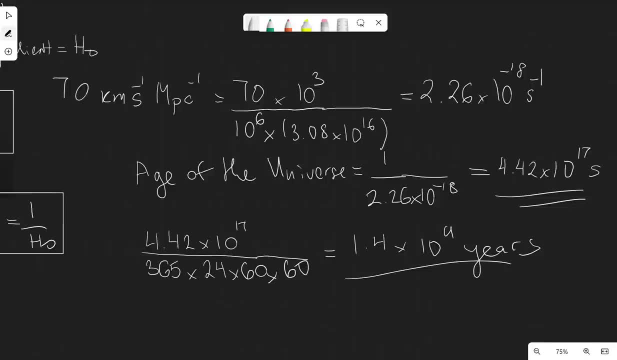 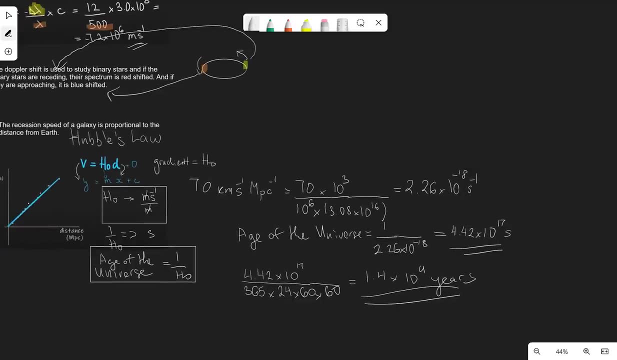 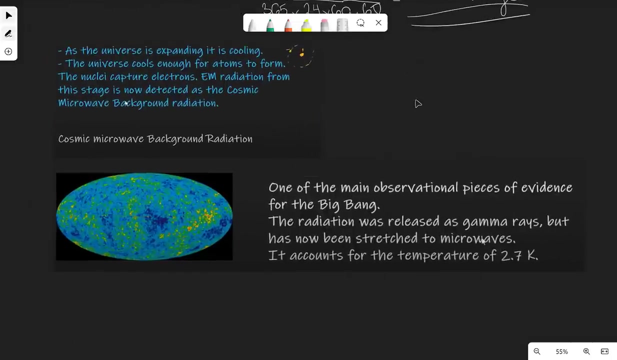 10 to the 9 years, and this here is approximately the age of the universe. please note that this here actually assumes linear expansion only. so this is an approximation. it's very, very close to the real number, but we need to say that it assumes linear expansion. so the universe is currently expanding and it is cooling. actually, it is expanding at an 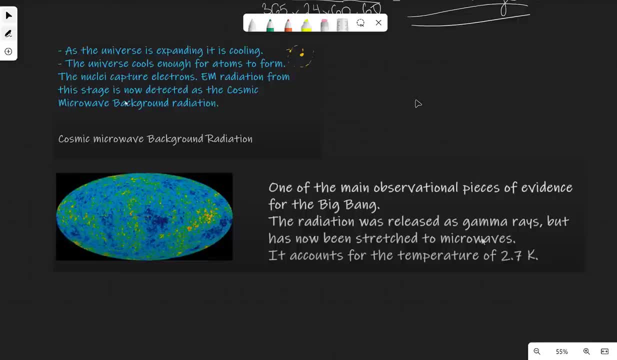 ever increasing rate due to something that we don't understand known as dark energy, but back in the early universe, as when it was expanding. eventually, the, the universe cooled down enough for the for the photons to break free during something known as the recombination period, when the electrons actually formed atoms and loads of radiation was created. 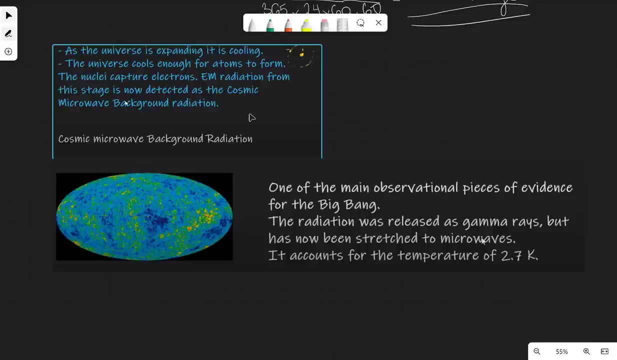 so this radiation has been continuously been stretched and not been released. we can say that the stretched with the expansion of the universe and is now known as the cosmic microwave background Radiation, and we've measured this and is one of the big observational pieces of evidence for the big bang. 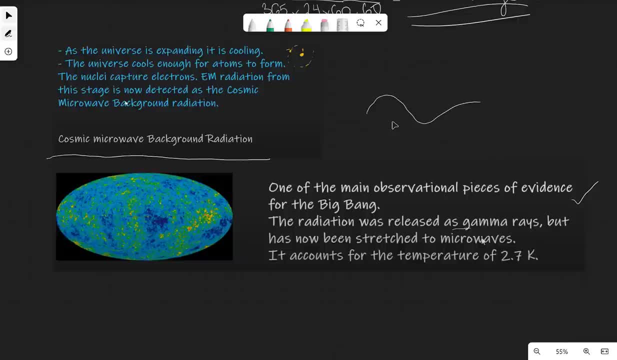 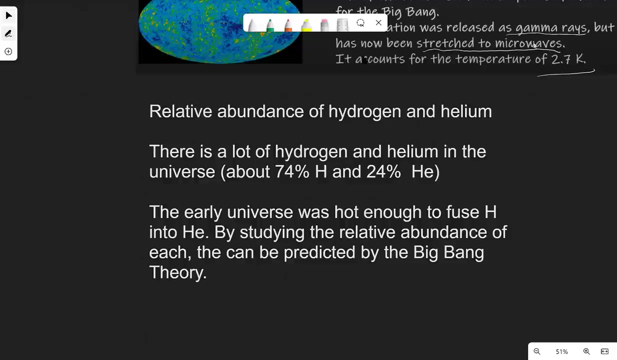 so this radiation was initially released as gamma rays, but has now been stretched to microwaves, and it accounts for about a temperature of 3.7 Kelvin. here's a picture from the WMAP space telescope of that radiation. Another observational piece of evidence for the Big Bang is the relative abundance of hydrogen and helium. 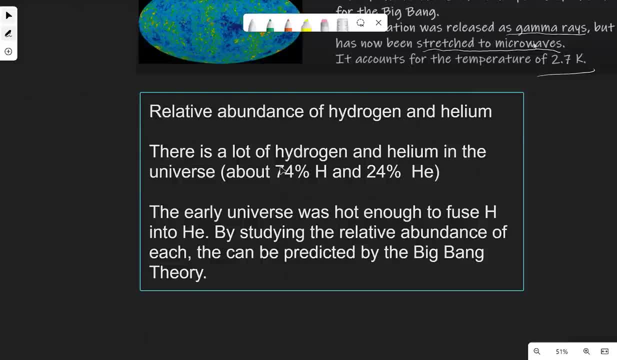 There's a lot of hydrogen and a lot of helium in the universe, more or less around 74% hydrogen and around 24% helium, and a couple of percent for all the other stuff. now, in the early Universe it was hard enough to fuse hydrogen to helium via nuclear fusion and we can actually predict by comparing. 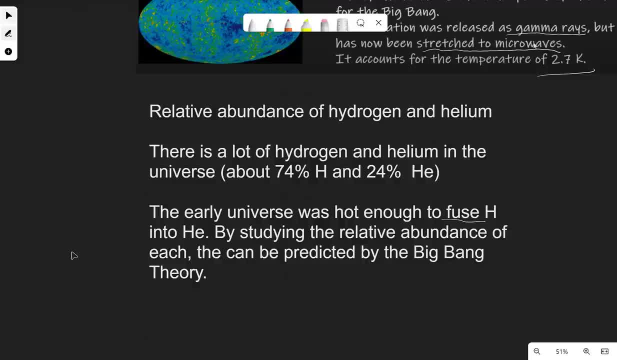 nuclear physics, that are relative abundancies of each of those substance substances, the proportions of how much this should be now and this matches the observational data, once again confirming what we know about the Big Bang Theory. and finally, we're going to revise briefly quasars, which are the most 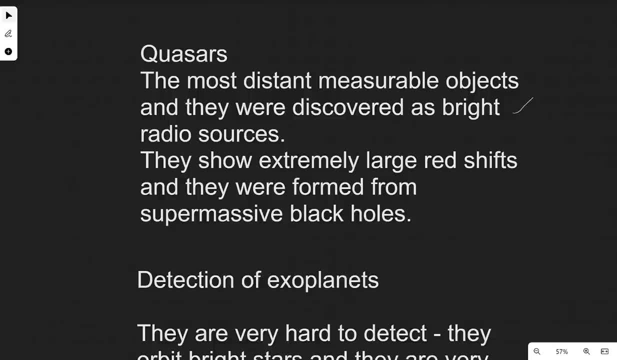 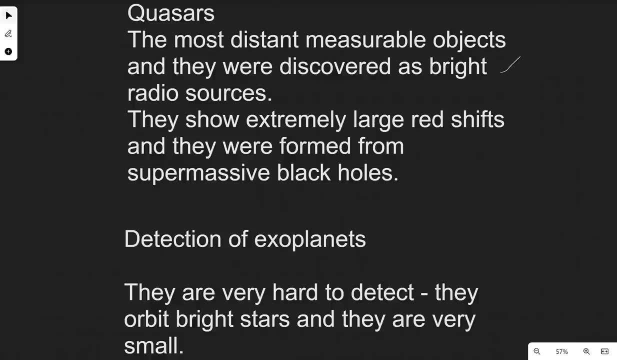 distance measurable objects. they were actually discovered as bright radio sources and they have the largest redshifts possible. they're these emissions as things aspiring, supermassive black holes, even the size of the solar system, with many, many, many billions of solar masses. really interesting objects, you. 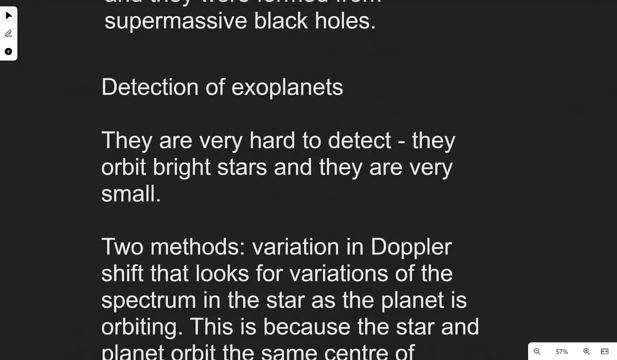 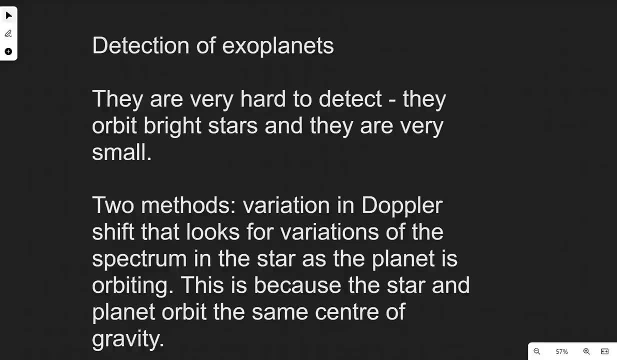 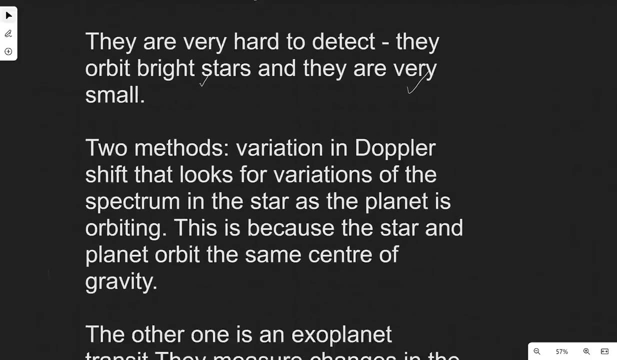 additionally, we're going to revise the detection of exoplanets, so these are planets outside of the solar system. they tend to be very hard to detect because they well, they orbit bright things, they orbit stars, and also they're very, very tiny. so if we're going to detect them, there's two methods. one of them is a. 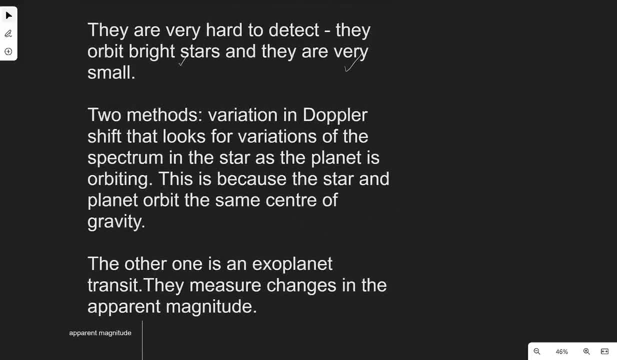 known as the Doppler shift method, and it looks for variation in the spectrum of the star. the planet is orbiting, orbiting, so some things might be getting a little blue shifted, a little bit red shifted, and vice versa. the change is tiny, though. it almost accounts for a small wobble of the star, and this is because the star in the